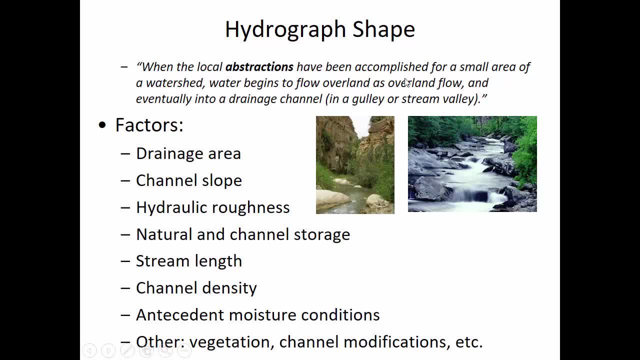 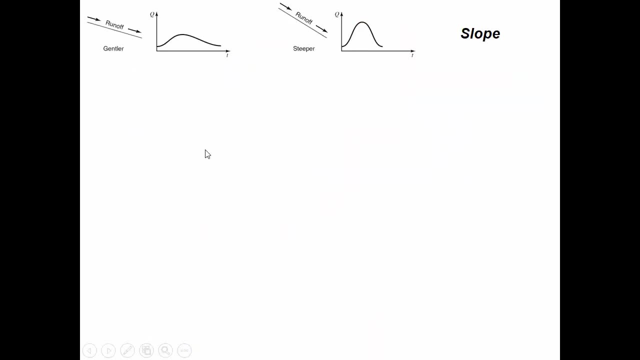 and the leaf litter on the ground, And so once all of that's done, then we can see overland flow starting to occur. And there are a lot of factors that influence how high the peak is or how wide the peak is on a hydrograph, And we'll go over some of these individually today. And so if you compare the effect of slope, what you'll see is that on relatively gentle slopes, where it's flat, the hydrograph 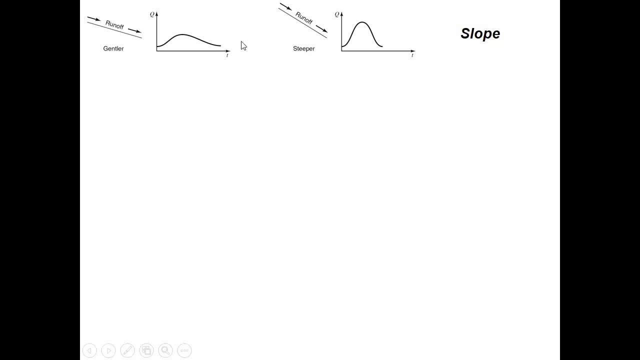 shape is more spread out And the reason for that is that the velocity as it travels over the surface is going to be higher for a steep slope And there's going to be relatively less of that diffusion effect that we talked about last time with the idea of pouring a cup of water into a flume and how it kind of spreads out the longer it's in the flume. So a steep slope leads to a higher peak and the peak is sooner than with the gentler slope. 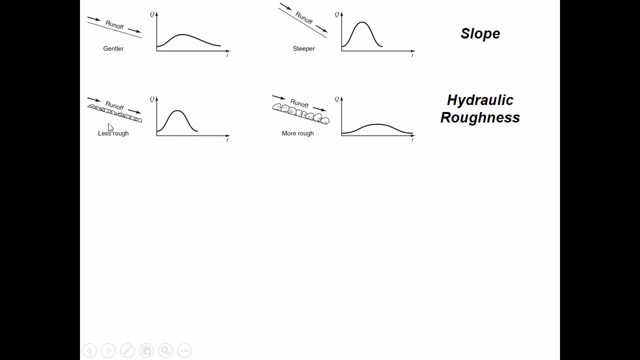 In case of hydraulic roughness, a surface that is smooth is going to tend towards a higher peak and a sooner peak, whereas the rough surface- with you know it's illustrated here with these big rock cobbles at the bottom of a stream- that's going to be slowing down the flow And because it slows down the velocity of the flow, it also tamp us down the the height of the peak. 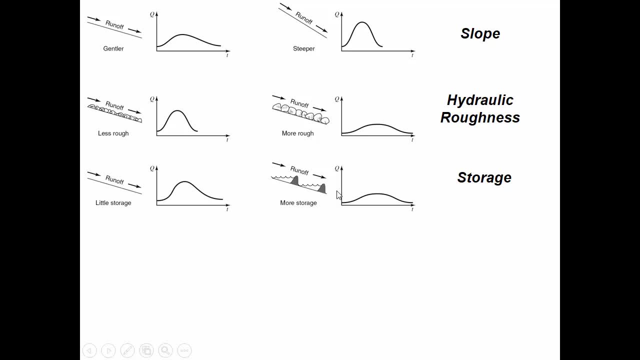 If we have storage in the stream, meaning for, for, for, For example, maybe an irregular cross section versus a relatively smooth cross section where there isn't any pools and ponds inside of the stream itself that have to be filled up before the flow goes down to the next pool or pond. 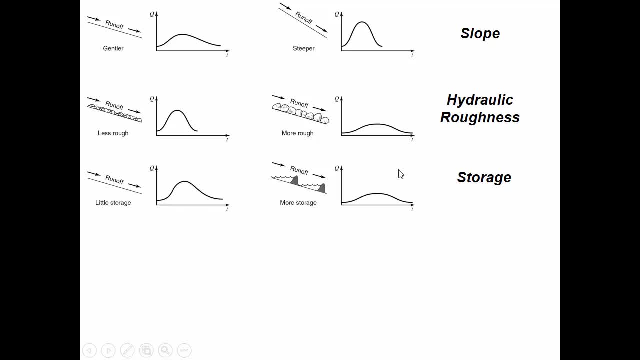 If there's little storage, then the peak is faster and higher compared to if each of these little. in a way, they're kind of like detention ponds inside of the stream that have to be filled up before the flow occurs. So this would be more akin to an engineered structure, an engineered channel, whereas 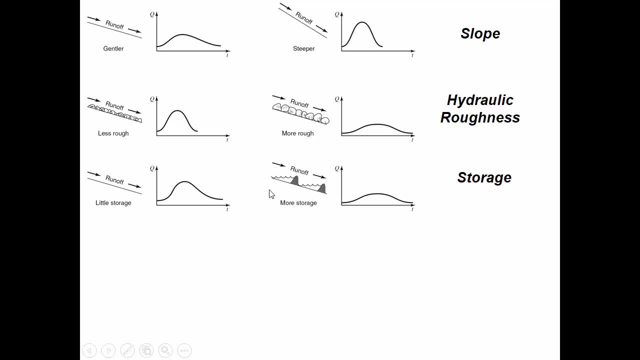 this would be a more natural structure or channel that hasn't been affected by human development. The drainage density is talking about how many secondary channels are feeding into the main channel in question. So if you have a lot of small streams and it's very easy for the oval and flow to 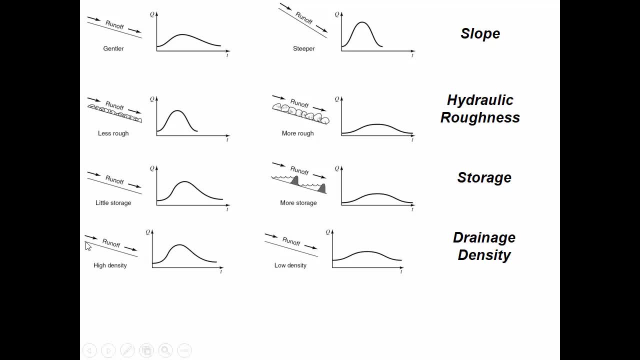 get into one of those small streams, then the high density of channels allows the water to travel over the land for less of the time, And so as soon as the flow gets into the channel, it's moving with a higher velocity. But if the water is going overland, then there's going to be a higher roughness value, a lower. 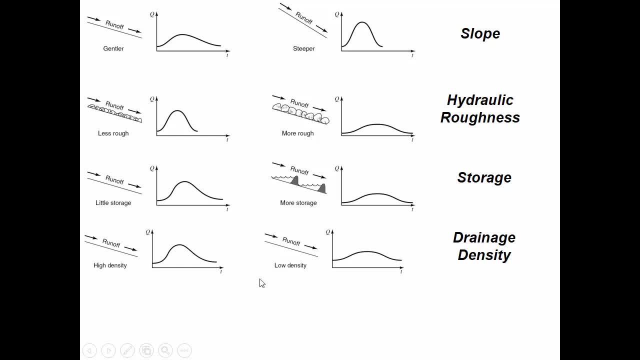 velocity, And so a low density of channels means that more overland flow and a lower peak, And finally, the length of the channel has an effect as well, Because even though the water is moving relatively fast in velocity terms, once it gets into, 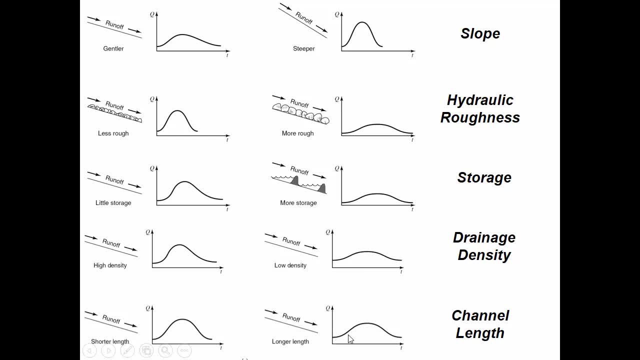 the channel. there's going to be a delay and more of that diffusion effect the longer the stream channel is, And so you'll see that some of these are more pronounced than others in terms of the effect that it has. The hydraulic roughness in particular can really have a big influence on how big the 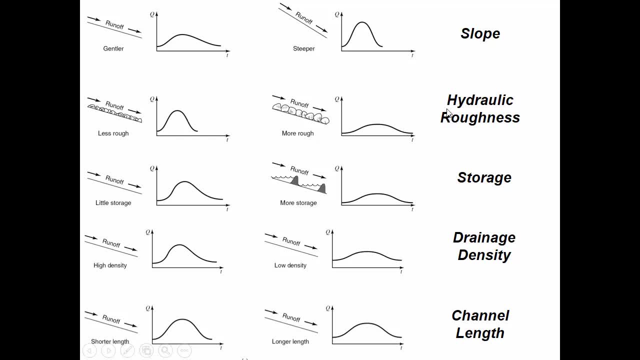 peak is going to be versus how spread it out. it is for a rough channel, Whereas in channel length it's going to be a little bit more. Yeah, It doesn't have an enormous effect on reducing the peak height and delaying it, And so all of these factors can be accounted for either empirically or they can be combined. 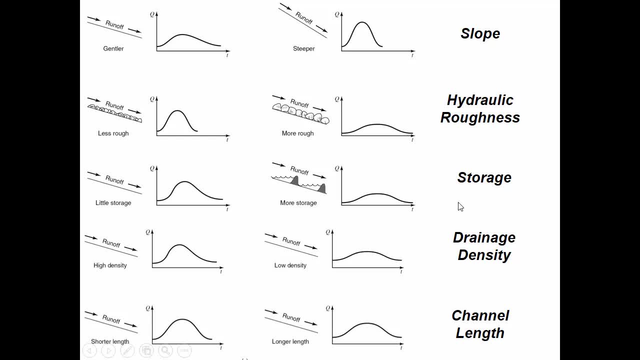 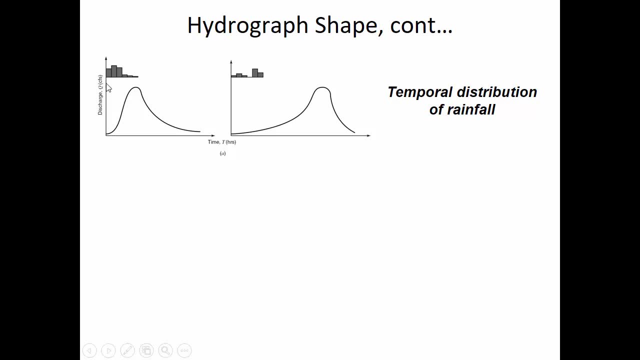 together in a unit hydrograph, which is what we're working towards discussing today. Here are just a couple of other considerations. If you think about the same amount of rainfall, but when in time it occurs, you'll notice that here It's a front loaded storm, where the intensity begins high and then it tapers off gradually. 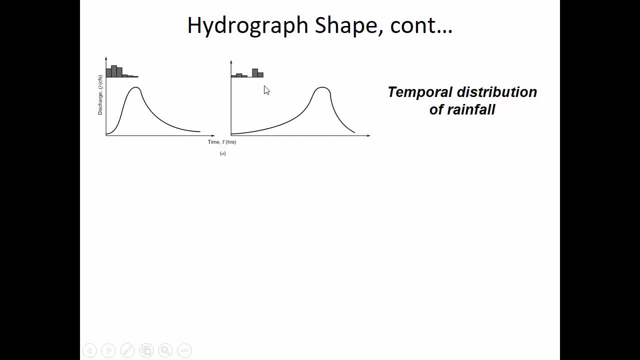 And what that's going to do is bring the hydrograph forward in time, compared to a storm that is back loaded, where more of the precipitation occurs later than the peak itself is going to be later, because the abstractions are overcome very quickly in the case of this, initially. 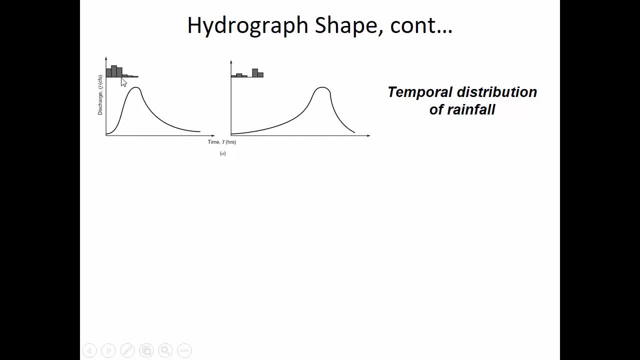 high intensity, But you'd think maybe it's not going to have as much of an intense effect as it ultimately does. These first few periods of rainfall intensity are just maybe barely enough to overcome the abstractions, And then we have to wait for some additional pulses of rainfall to come through before 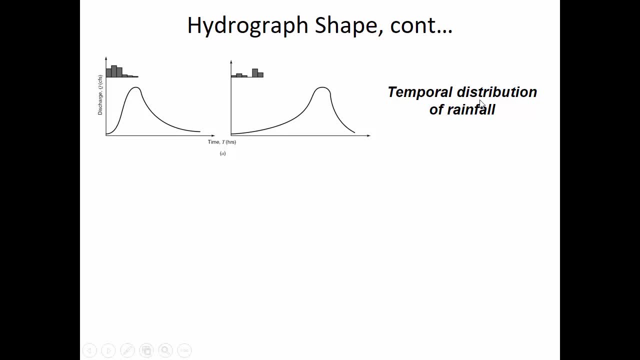 the hydrograph actually begins to take shape, And this idea of looking at when, during time, certain things occur, that's called temporal distribution, And so there's a difference between temporal distribution and spatial distribution. Spatial distribution is looking at where in space there may be variation in intensity. 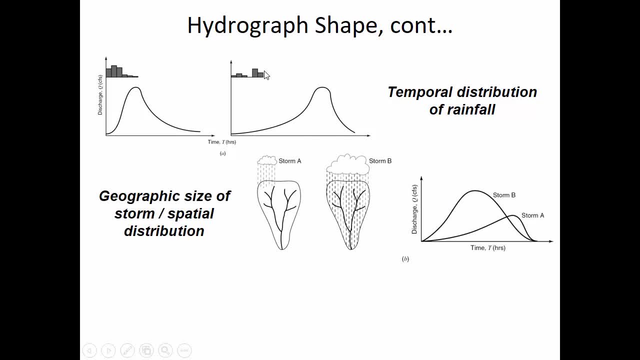 Temporal distribution is when, during time, is there variation in intensity. And so this next figure is an illustration of variation in spatial distribution. And so it's showing, for instance, that if you have storm A, which is just falling on a certain fraction of the watershed, then that hydrograph is going to be not only lower, 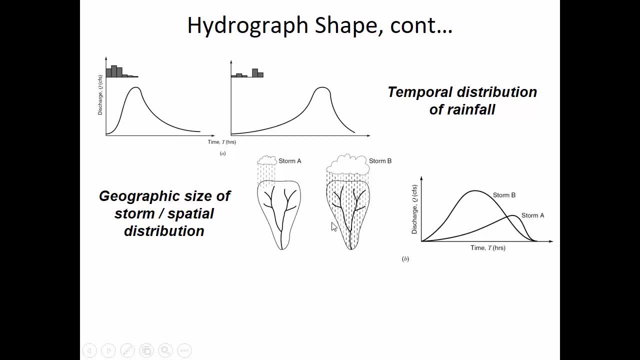 but later. Because what storm B does, when the water's falling over the entire watershed, is that the channel is becoming wet with the flow. Let me just point on the whiteboard here. So the flow that gets into the channel from here wets this segment of the stream so that 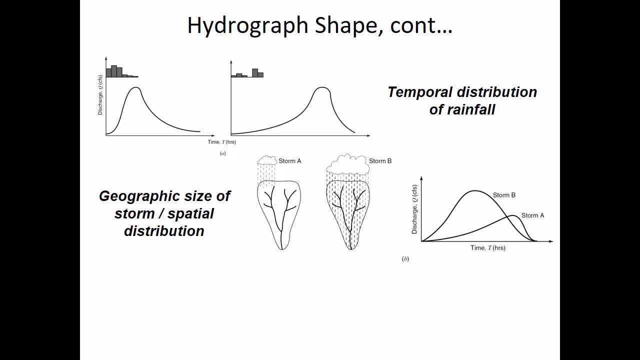 when all of the watershed is finally contributing, when the time of concentration has occurred and the entire watershed is contributing to flow. All of the stream has been wet in advance of that, Whereas in the case of storm A, it's just this one slug of water that has to first of 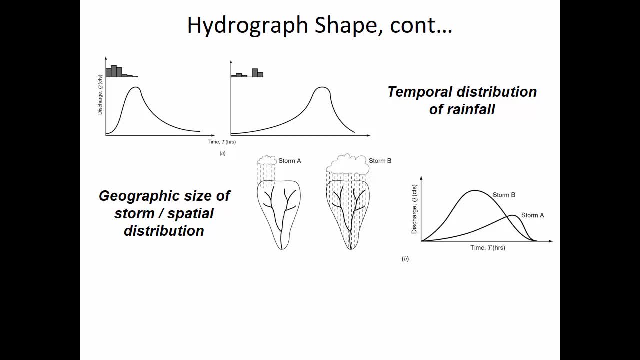 all travel overland, And then, as it's traveling through a dry channel, part of the flow is being stuck to the surface and lagging behind as it wets the bottom of the stream, And so there's a pretty pronounced lag and decrease in volume effect because only a fraction. 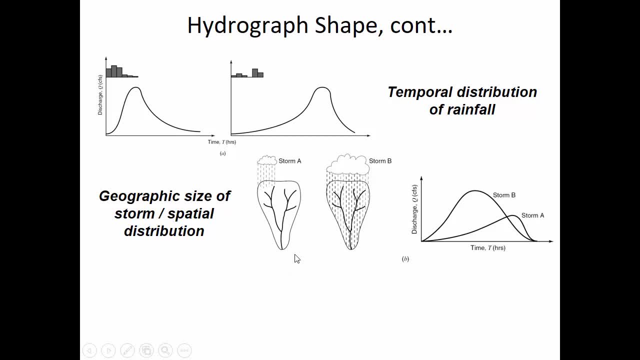 of the watershed had rainfall, And so, depending on where your rain gauges are, if you had a rain gauge in the section of the watershed that is experiencing the storm, you may assume that it occurred everywhere, And so there can be a lot of variability that actually isn't seen, depending on where you. 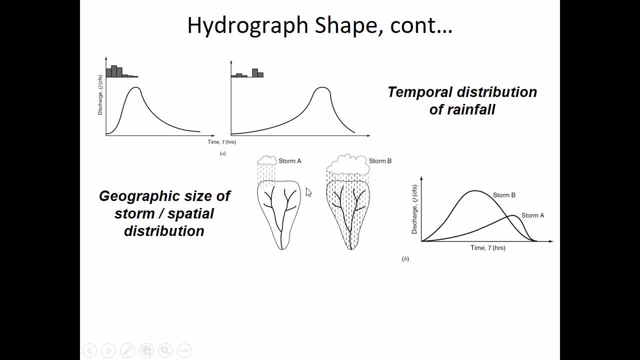 have your rain gauges, And so it may look like the entire watershed is experiencing a storm, but then if you were monitoring the outflow at this point- Okay, At the outlet- you'd be puzzled as to why you had such a small hydrograph compared to. 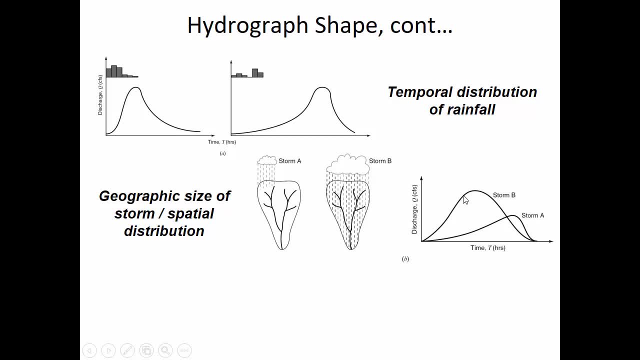 previous storms that were measured, And so you see nowadays increasing emphasis on radar being used to characterize the storm coverage, rather than relying just exclusively on rain gauges that are at a single point. They're starting to use these radar cells 2.5 kilometers by 2.5 kilometers, and trying. 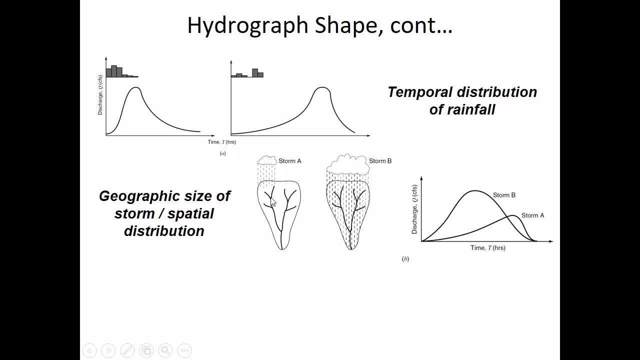 to estimate how much precipitation there was. Okay, And so you can see that this is a very high resolution. This figure from the book kind of illustrates the effect of storm movement, And that is if it starts raining at A and the wind is blowing the storm towards B. so 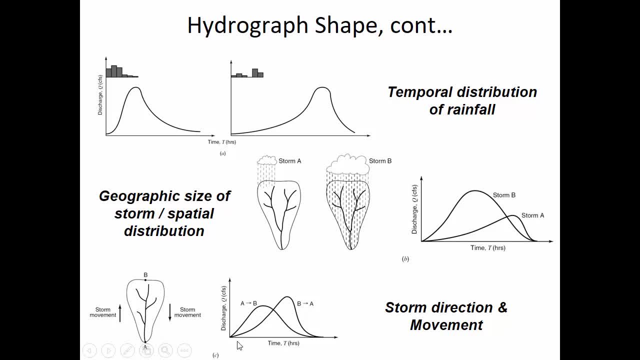 if the storm is moving away from the outlet, then what happens there is that it occurs much more soon than if the storm begins at B and is working towards the outlet. And so if the storm is beginning at B, then it's moving towards the outlet. 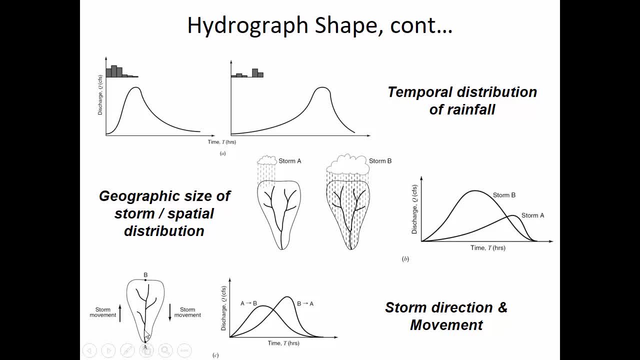 And so if the storm is moving towards the outlet and it's working towards the outlet, then then the rest of the, the channel, hasn't been wet in advance, in advance. and if the channel is wet in advance, then that brings it, shifts it forward, but you'll notice that the amount is higher in. 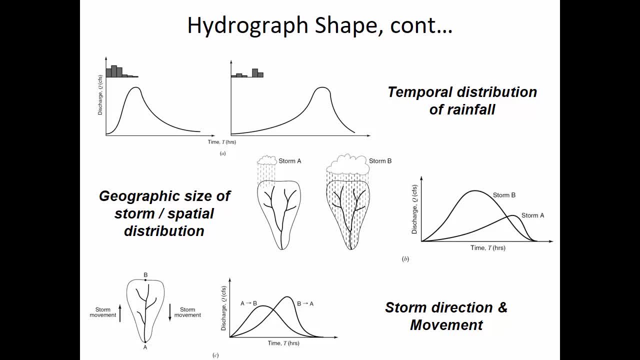 the case of b to a, because the rain is kind of following the movement of the storm, as the water in the channel is moving downstream, so it's raining on top of that and so it's kind of bringing it all together at the same time, and so the peak is higher, even though it's delayed. so these are just. 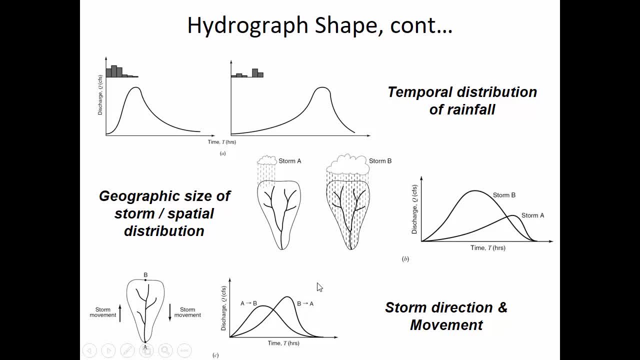 some of the physical effects that we have to ask when we're looking at storm data is: you know where in the watershed was the storm? over what time period was it maybe even through the entire duration? or was it front loaded or back loaded? so these are important physical effects. 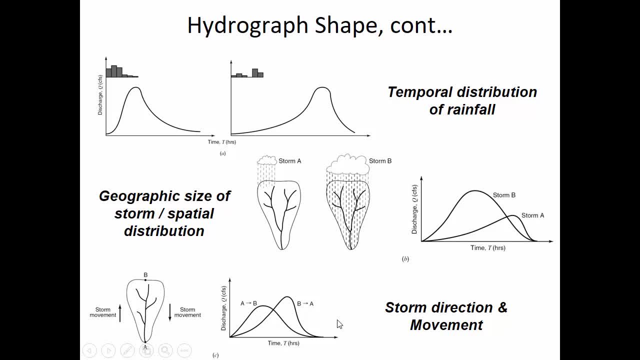 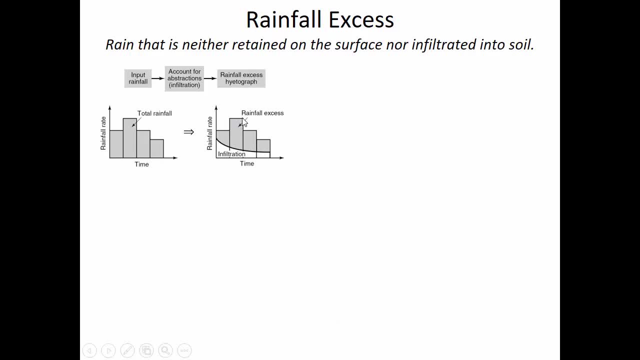 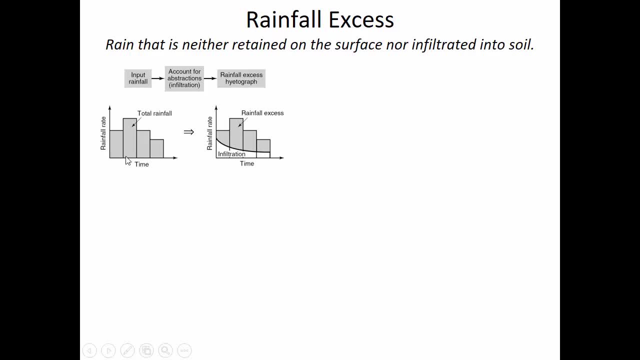 hydrograph and it's showing a graph of time and rainfall intensity. you see, it's broken up into time segments and so we've got some variability in the rainfall intensity over time. this is the typical declining rate of infiltration. um ok, why does soil infiltration rate decline over time? 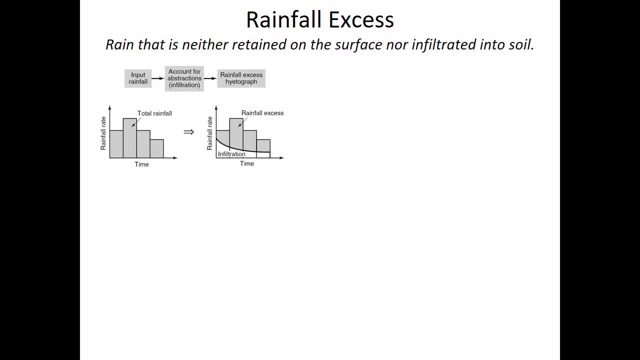 Why is it getting lower, Jeffrey Well, ground has absorbed too much water and it can't take any more in it. Ok, why not? Why, when the ground has started to absorb water, why does the infiltration rate decrease? Suction pressure. 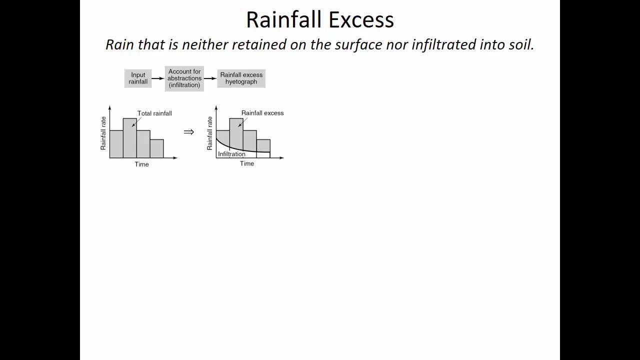 Suction pressure. Remember that the suction pressure on the ground is going to be reduced as it's absorbed by water. Ok, When the suction pressure is high, that potential attraction that the soil has for water is high when the soil is devoid of moisture. 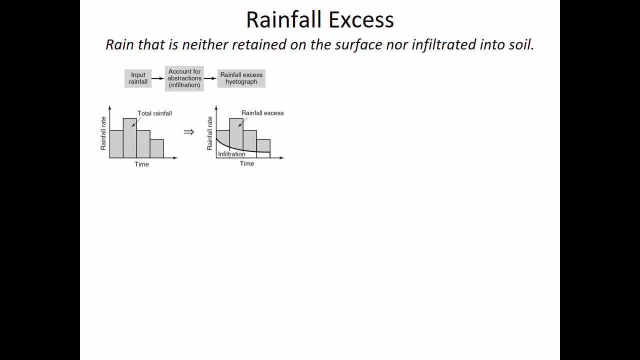 But as more of the voids get filled up, then the suction pressure decreases, and so then what's left to drive the soil downward is just gravity and maybe pressure from above, where the main effect early on was that the soil itself is drawing the water downward. 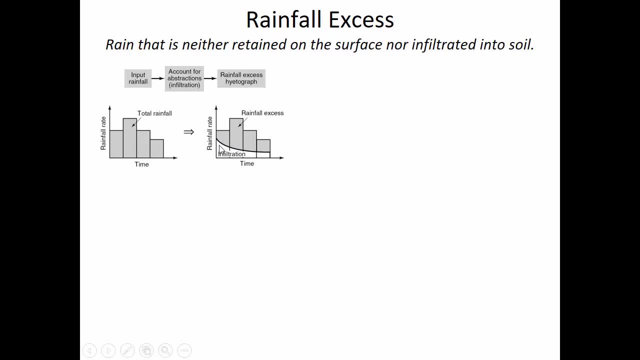 It's kind of sucking it down from the surface Over time. what this is showing is the declining rate of infiltration. so anything above that curve we call rainfall excess. So it's the excess that's above and beyond the abstractions and infiltration. 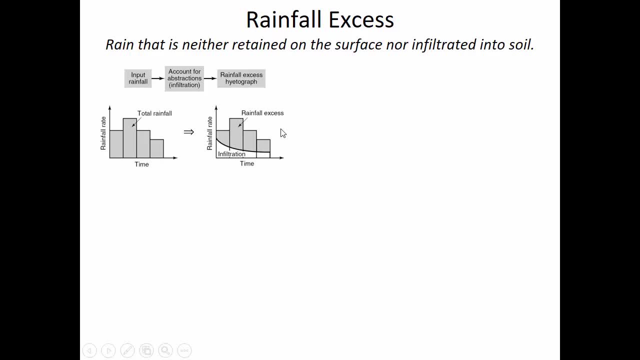 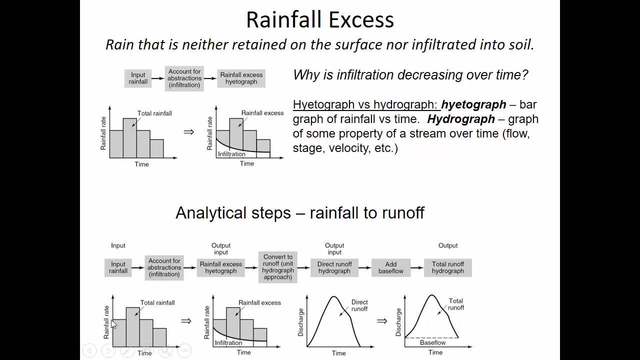 And so rainfall excess is what contributes to outflow from a watershed. So we've talked about why infiltration decreases over time. A Hieto graph, remember, is a rainfall intensity figure, Whereas a hydrograph is a runoff figure. Now, what we want to do is connect the dots between measuring rainfall. 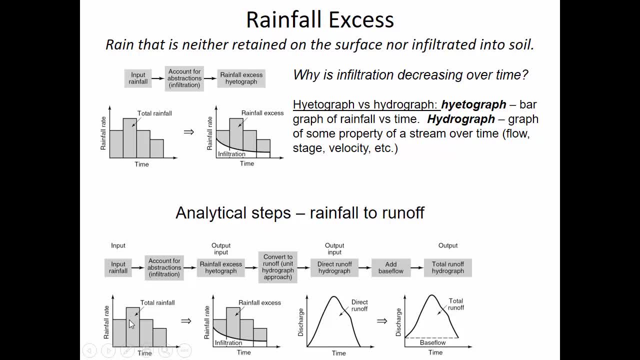 knowing how much of that rainfall is going to be abstracted, meaning surface wetting mostly- how much of the rainfall is going to be infiltrated, because the difference between rainfall and the abstraction and infiltration is rainfall excess. So we've talked about 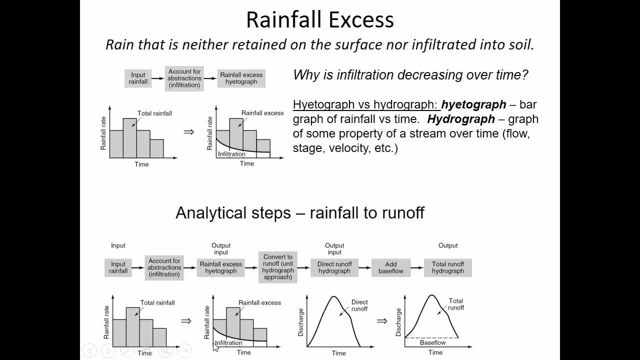 equations that you can use to estimate infiltration. Remember there was the Horton equation, There was the Green-Ampt equation. So we have some numerical tools that will tell us this infiltration curve. And we've talked about where you get rainfall data. You can get that either from a rain gauge or from an intensity-duration-frequency curve. 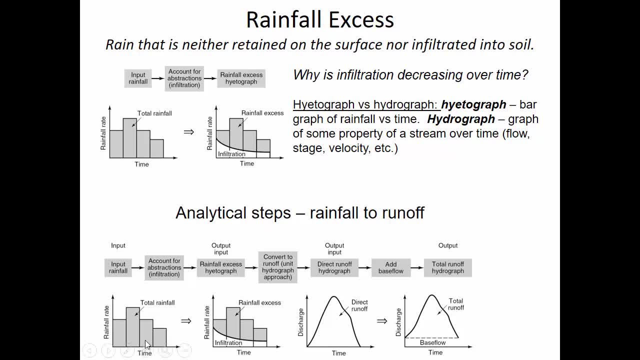 So we have real-world sources of rainfall data. Rainfall excess is just going to be the difference between them, But what we need now is some way to predict what the shape of the curve that comes out of the watershed looks like, And the method we're talking about today is a unit hydrograph. 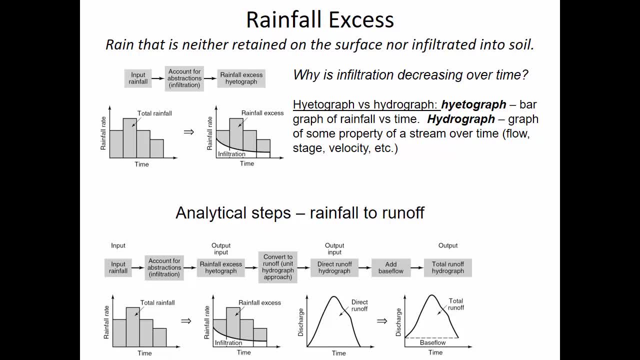 And what a unit hydrograph does is it says, for a certain amount of rainfall excess, we expect a typical shape of the runoff out of this watershed, And if it's a big watershed then the runoff hydrograph will have a different shape. 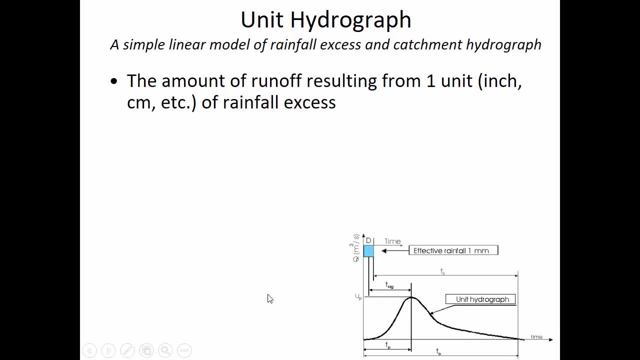 characteristic shape than a small watershed would. So here is a typical runoff hydrograph that's occurring from a unit of rainfall, And we call it a unit hydrograph because the idea is that if we have a certain amount of rainfall excess, whether it be an inch or a centimeter- 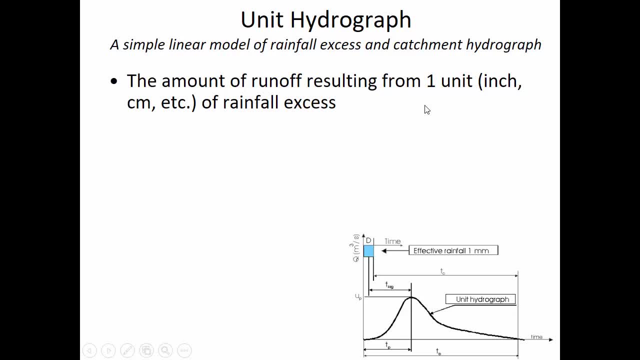 we could prepare a relationship like this for any particular unit of rainfall excess. We want to know, for a watershed in question, what does the typical curve of runoff look like? So you're assuming uniform coverage over the watershed, So it's not just for a certain part of the watershed that's having rainfall. 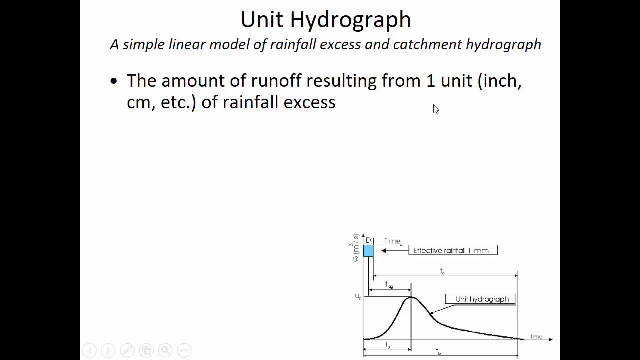 You'd want to know if you had one inch of rainfall excess, meaning that you've accomplished- Excuse me, Coronavirus- If you have accomplished the abstractions and infiltration has been satisfied. so an inch of rainfall excess, what is the typical curve look like? 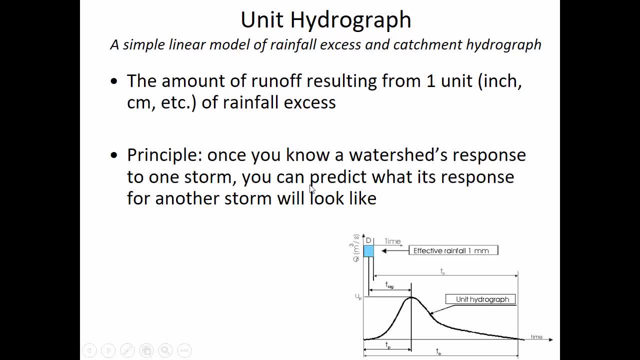 The idea is that if you know what the watershed does for one inch of rain, then you can scale it linearly. for two inches of rain, You've just doubled the hydrograph, And I should be really precise as I'm speaking, If you know the response for one inch of rainfall excess. 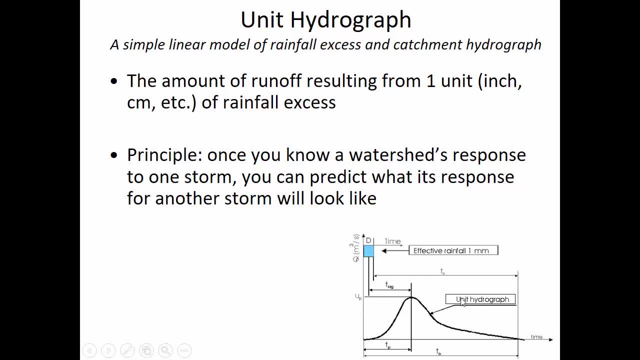 then you can linearly scale the response to two inches of rainfall excess, And so we're not talking about that. the hydrograph isn't in response just to one inch of rainfall, It's to an inch of rainfall excess, And so it's just the stuff that's left over after all the other taxes. 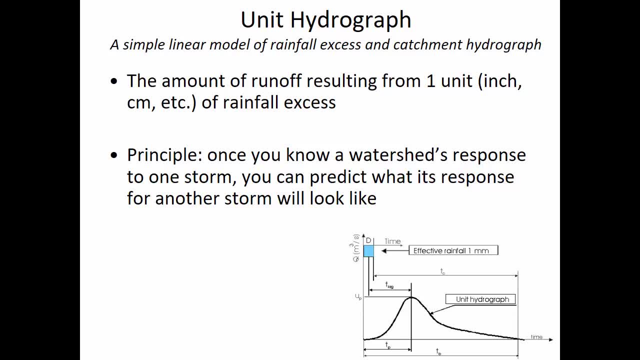 maybe you'd think of them on the rainfall itself, The things that decrease the quantity of rainfall that's going to be running off. So there are some assumptions to applying this simplistic method And with the unit hydrograph you'll notice that we're assuming that the pulse of rainfall has a constant intensity. 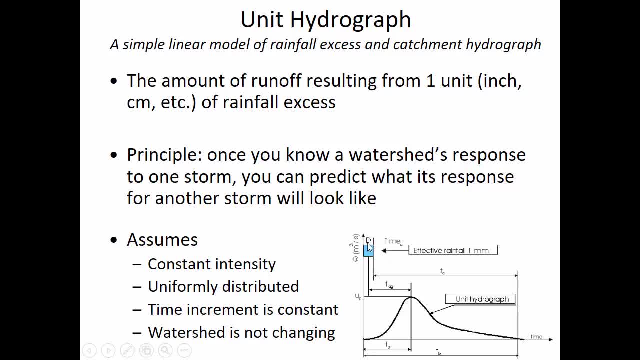 during this unit of time and unit of depth, And we're assuming that it's uniformly distributed over the entire watershed and that the watershed isn't changing over time, And so to apply this unit hydrograph, you'd assume that there are no seasonal variations. 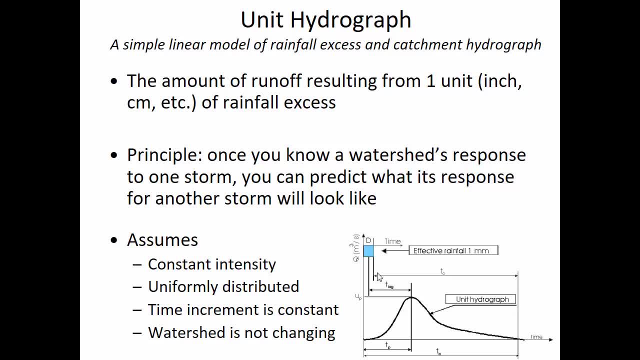 which, of course, we know that there are, And so the way you'd correct for that is maybe you'd have a summer unit hydrograph and a winter unit hydrograph. So this is: how does the watershed respond as conditions change? But if you have this unit hydrograph, 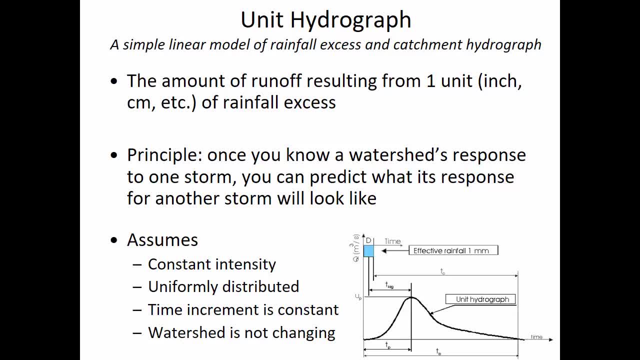 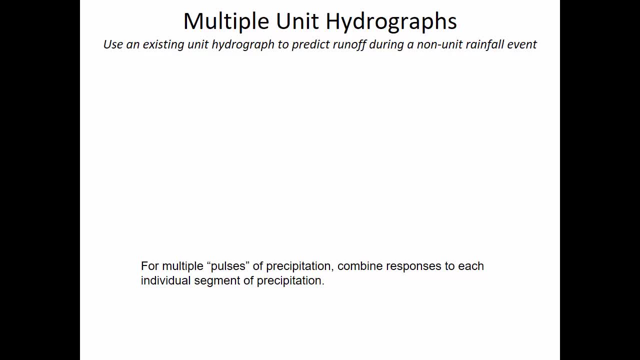 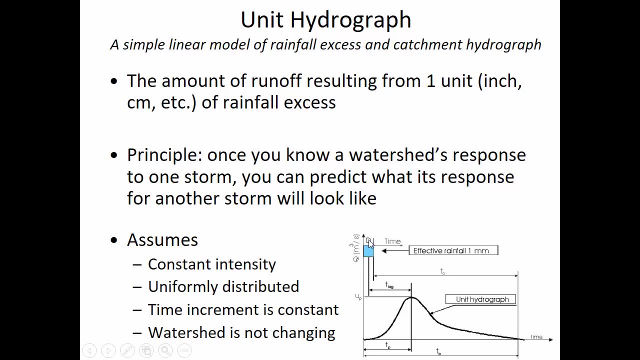 it allows you to extrapolate for any kind of storm regardless of duration or amount. Now the thing that's a little bit tricky is when you do have a storm that is a longer duration than this single unit duration. So this might represent it's saying here: 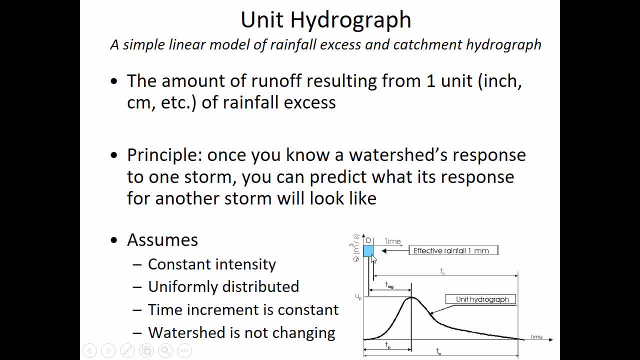 one millimeter of rainfall excess, And let's assume that that's an hour of duration. What if you had a storm that lasted three hours of duration? What we would have to do is we would have to set it up with overlapping curves, And then the effect is additive in combining the watersheds together. 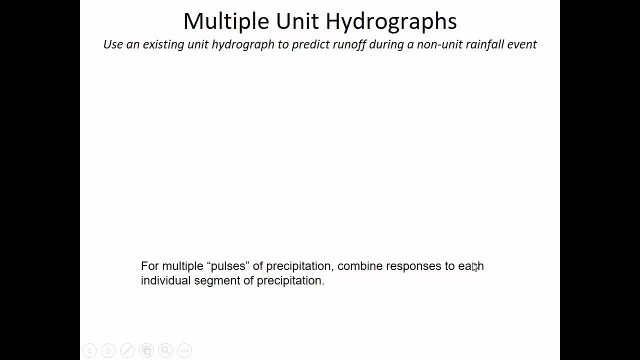 So if there's multiple pulses of precipitation, we combine the responses, So you'll be given a certain amount of precipitation during a certain time period And you'll know the unit scaling response And we want to know what's the runoff for that one particular period. 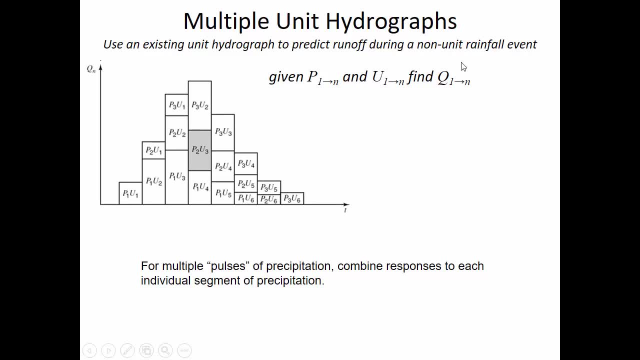 But then there's going to be precipitation from other periods as well, And so there's this figure from the book that shows the formula that would be used for a storm where you have three different precipitation amounts. So you'll notice there's P1, P2, P3.. 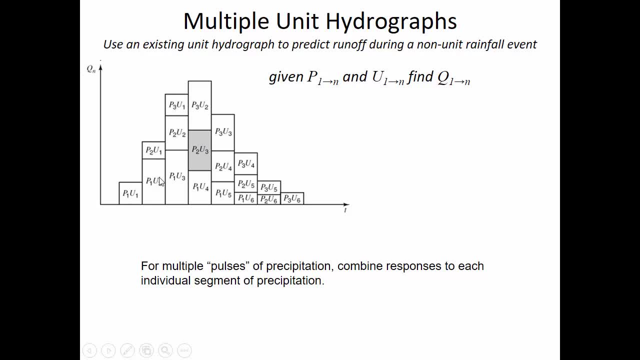 And then the U here is referring to what the watershed does during the first hour, the second hour, the third hour. So this formula probably doesn't make a lot of intuitive sense yet, But it will when we start doing things with the spreadsheet. 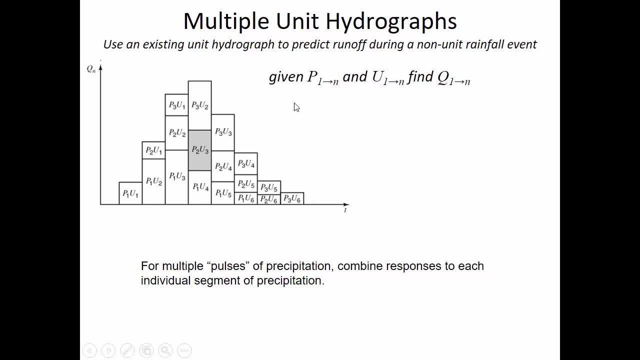 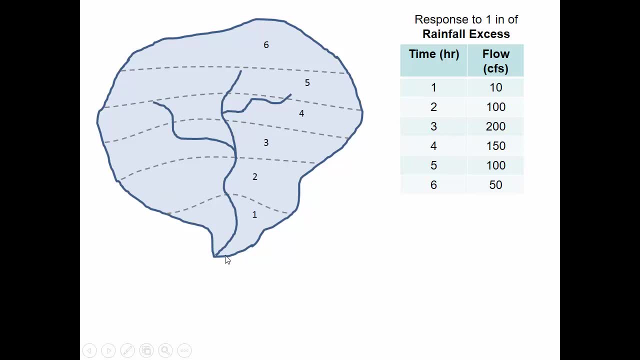 You'll look at what's happening with the spreadsheet And then we'll take another look at this figure And I'll illustrate what this figure means. But the idea is that here is just a sample watershed And these numbers 1,, 2,, 3,, 4,. 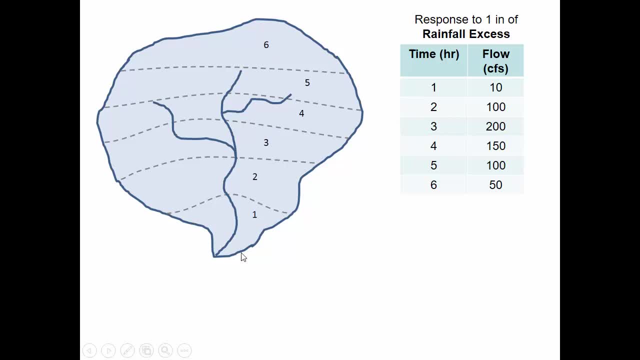 what this represents is the amount of the watershed that's contributing to the outflow in a given hour. So in the first hour, if it's raining over the whole watershed in the first hour, it's only this area that is contributing flow at the outlet. 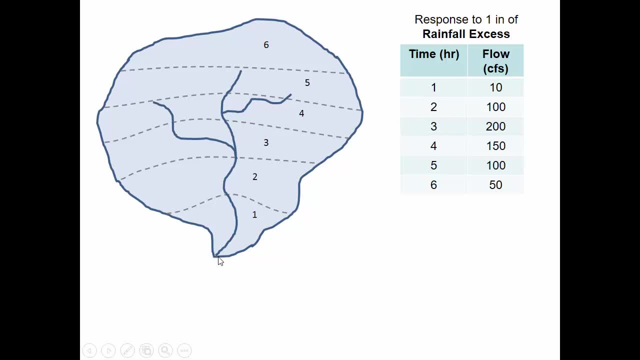 because of travel times, And so after two hours, then, finally, you're getting the water that fell in this area, This region too- at the end of the second hour, that's contributing to flow. At the end of the third hour, finally, this area is contributing to the outflow. 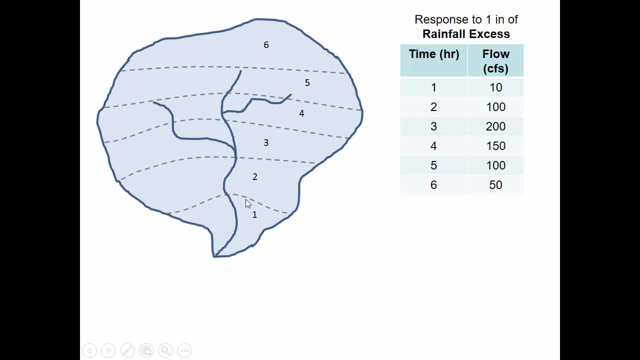 So these time bands are kind of working further and further away from the outlet. Now, this is the response to what happens if there's one inch of rainfall excess in this watershed, And so what this is showing is that, if it rained over the entire watershed, 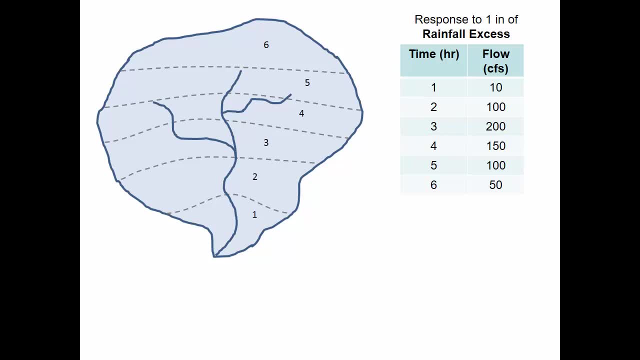 for one hour. so the rain duration is just one hour and the amount of rain is such that there's an inch of rainfall excess. So there was more than an inch of rain. There was an inch plus the amount that's going to be required for infiltration. 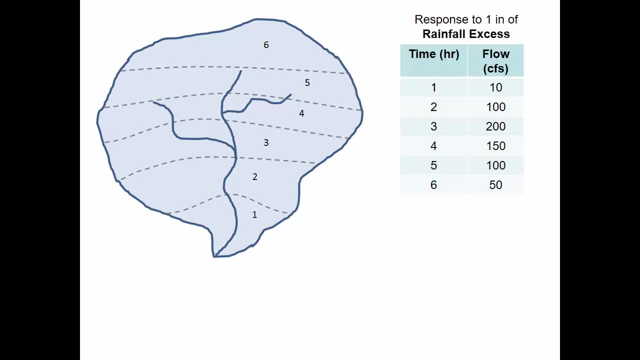 plus the amount that's going to be required for abstractions. So there was enough rain that there's an inch of rainfall excess, And then what comes out of this particular watershed is this hydrograph, And so the time is more than an hour, because the rain that falls all the way out here. 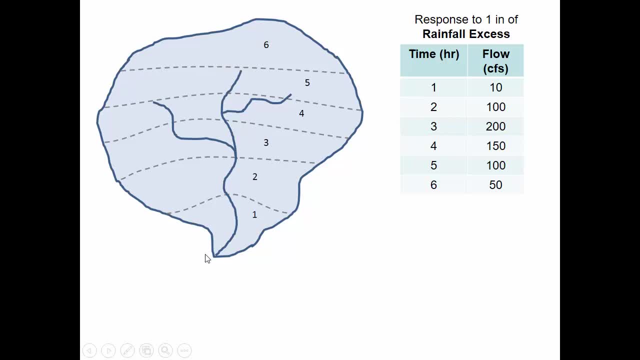 is going to take six hours to travel to the outlet. And so what? we see this 50 CFS. that's still the rain that fell during the zero to one time period during the first hour, but it's just it's taken so long to finally make its way to the outlet. 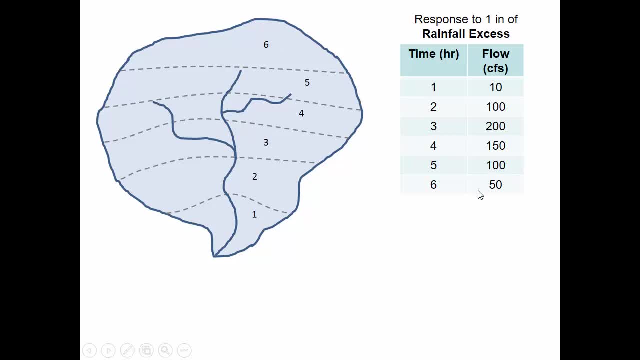 So that's why we only see it at hour six is because of the lengthy travel times through the watershed. So just to say it one more time: this is the response to a storm that occurs in just one hour From time zero to time one is when the rainfall excess occurred. 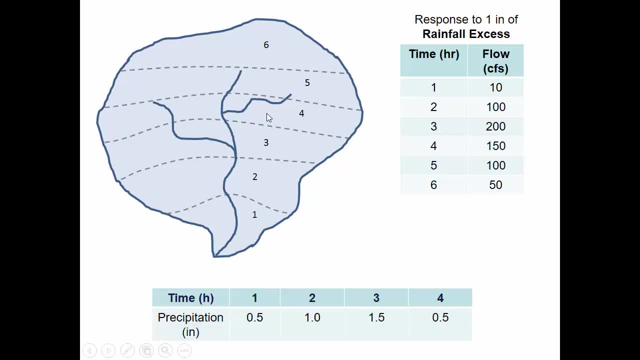 and then we have it draining the watershed over six hours. So the question is: what if we have a storm that's more than a single hour? What if we had a storm that in the first hour there was 0.5 inches of rain? 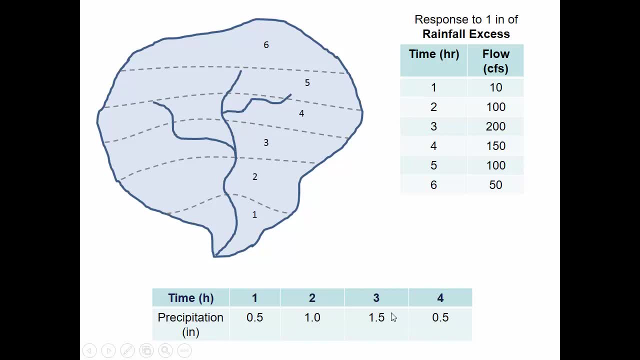 In the second hour there was an inch, The third hour inch 1.5. And in the fourth hour, 0.5 inches of rainfall. Then what would the hydrograph look like? And so that's what we're going to do with this template file that I've provided. 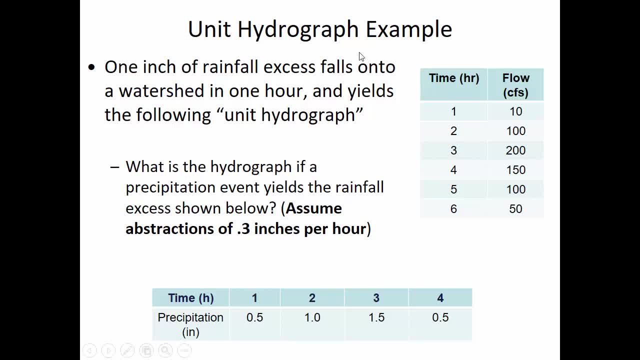 So if you haven't already downloaded it in Excel, go get that template file, because what we're going to do is go through the process of creating a staggered unit hydrograph. where there's an inch of rainfall excess that gives us this unit hydrograph. 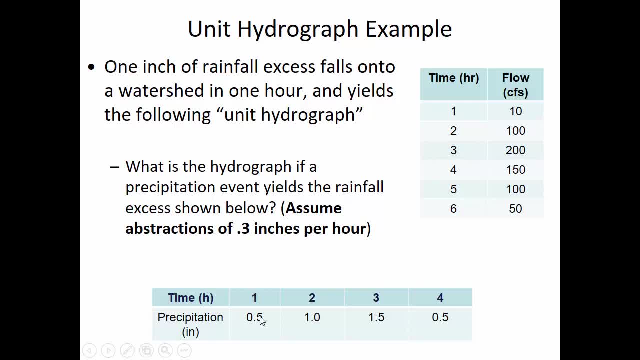 and then we know the precipitation amounts and we're going to reduce them with the assumption that there are abstractions of 0.3 inches per hour. So, just for purposes of simplicity, we'll set aside infiltration for now. We'll combine infiltration and abstractions together. 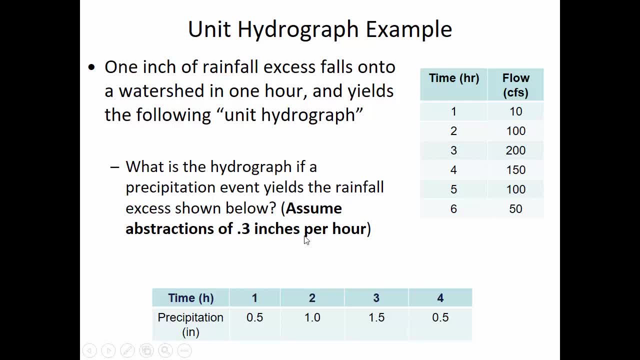 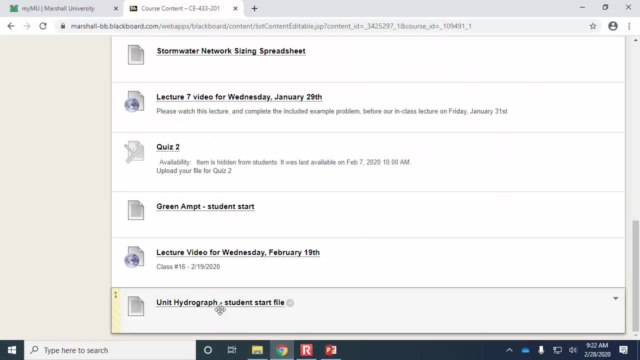 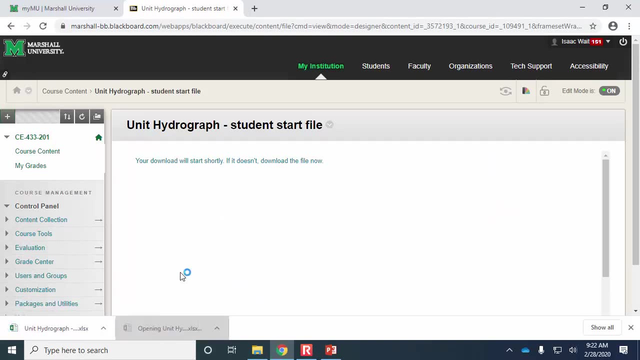 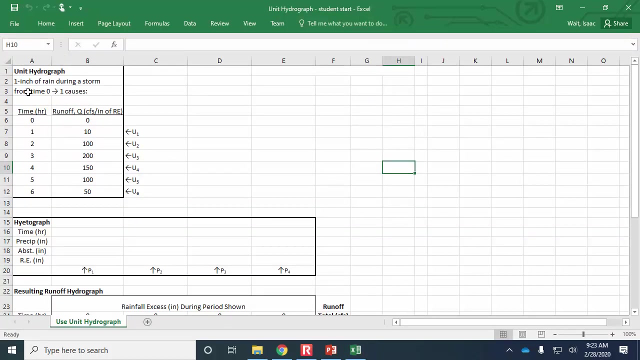 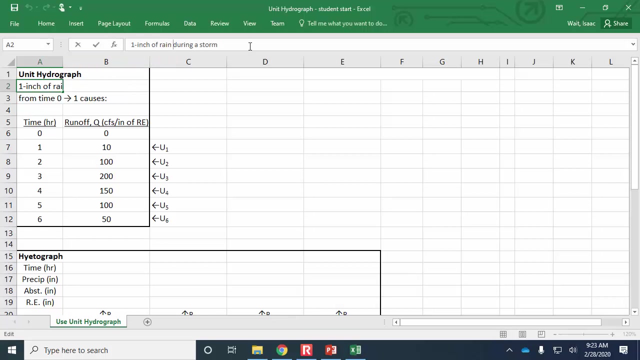 and assume it's linear, just so you can see the unit hydrograph part of it. Okay, so here is the student start file that we'll utilize. All right, so here it's, reiterating that if you have an inch of rain, 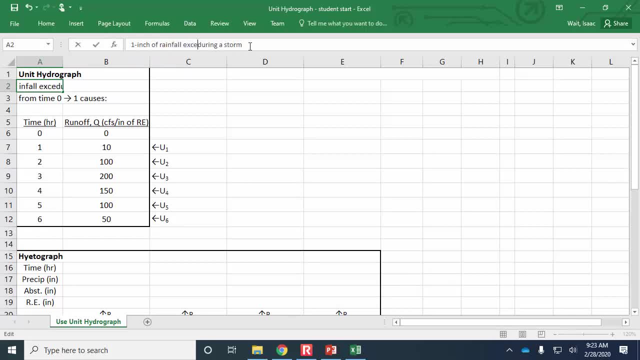 Let's change this to make it so precise: Rainfall excess is what is causing this: An inch of rainfall excess, the period was from 0 to 1, and that inch of rainfall excess was a constant intensity over the entire watershed, then this is the response that we get. 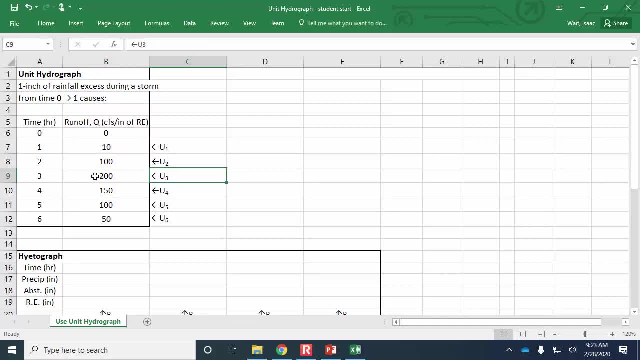 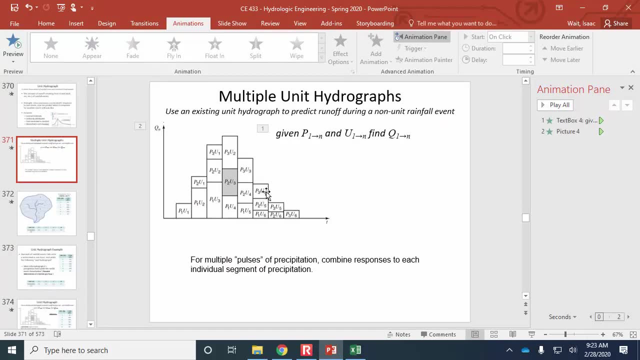 And we're calling this U1,, this U2,, this U3, and those designations correspond to this kind of a figure. So it's not important to just from the spreadsheet perspective to label them, But when we go back and compare the results we get to this figure. 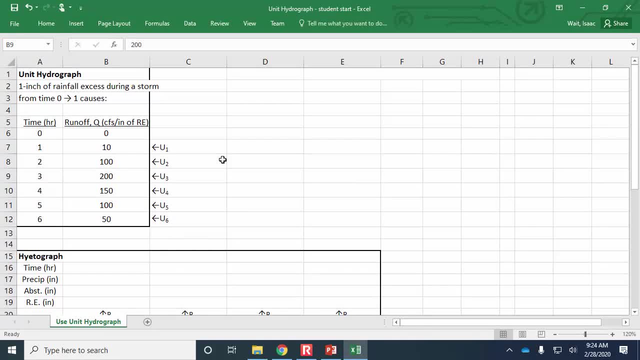 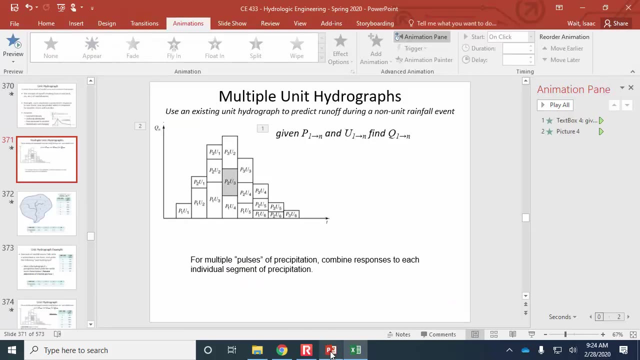 I want you to know that the U1 is basically the unit response during the first hour, the unit response during the second hour, the unit response during the third hour, And so forth. Okay, so now, here in this hydrograph window, we're going to transfer the data that we have in the problem statement. 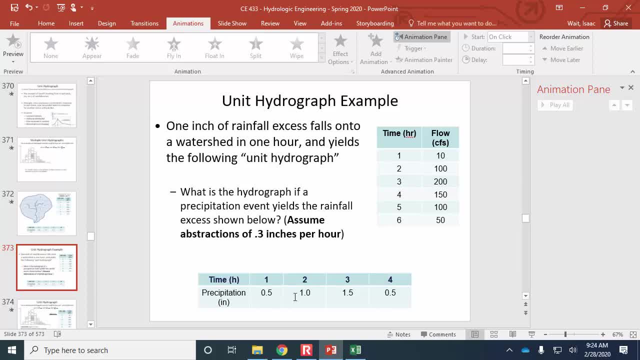 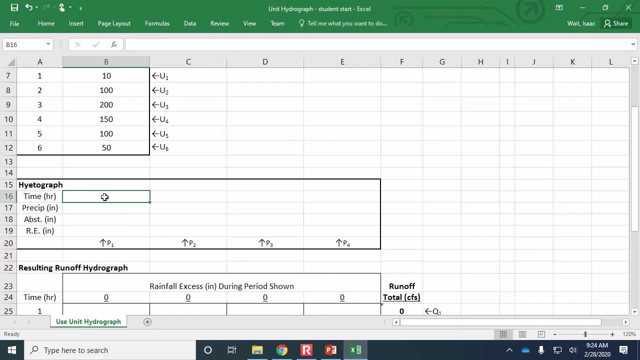 So time 1,, 2,, 3, and 4, we know the precipitation amount and we're going to reduce out the abstraction to find out how much rainfall excess is left. So it's during hour 1,, hour 2,, hour 3, and 4.. 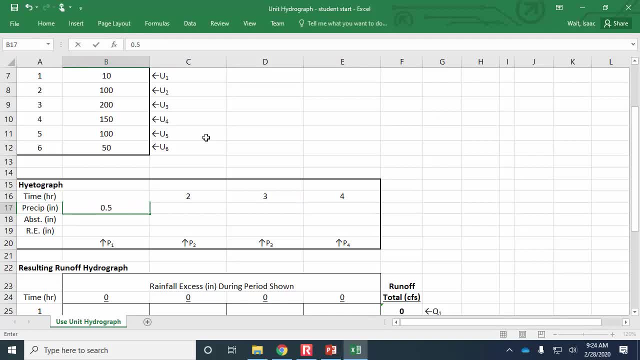 The precipitation amounts were 0.5 inches an inch 1.5, and 0.5.. And for this illustration we're just assuming constant abstractions of 0.3, but in reality, if you were doing this a little bit more sophisticated, 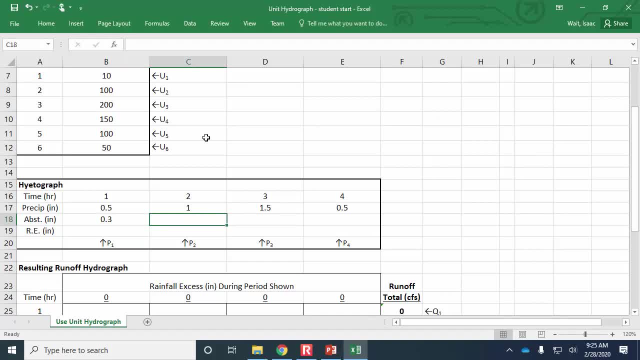 what you'd try and do is apply the Horton method or the Green Amp method and find out what is the declining rate of potential rainfall, What is the declining rate of potential infiltration during each of these time periods, And so you'd say how much infiltration was there in hour 1 of the storm. 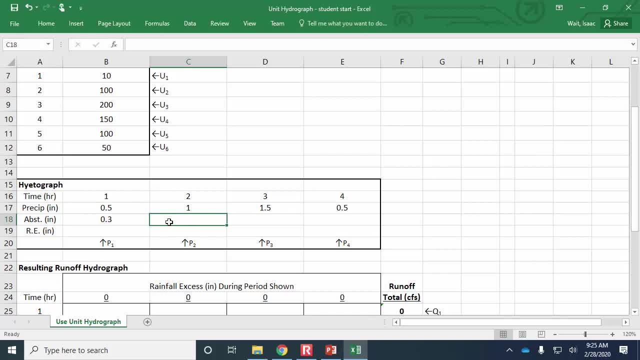 in hour 2 of the storm And you'd actually calculate the amount of abstractions rather than just using this placeholder constant value. So rainfall excess is precipitation amount minus the abstraction. So 0.2 inches during the first hour, 0.7 during the second. 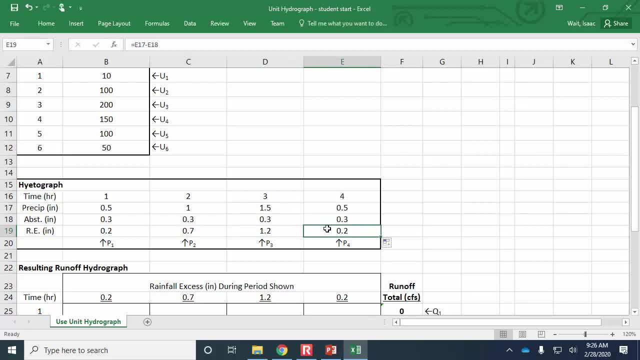 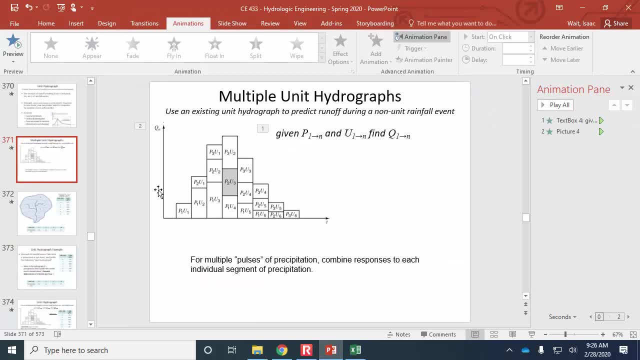 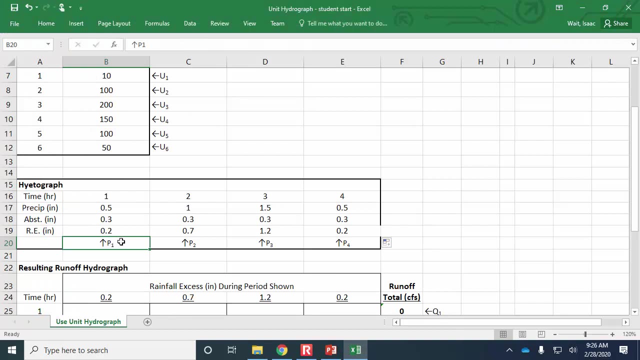 1.2 in the third and 0.2 in the fourth. So back to this figure that we're going to be looking at: P, P1, P2, P3. That refers to the precipitation amount during the first time interval. 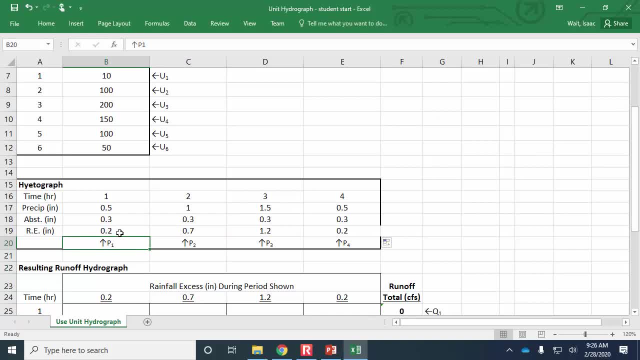 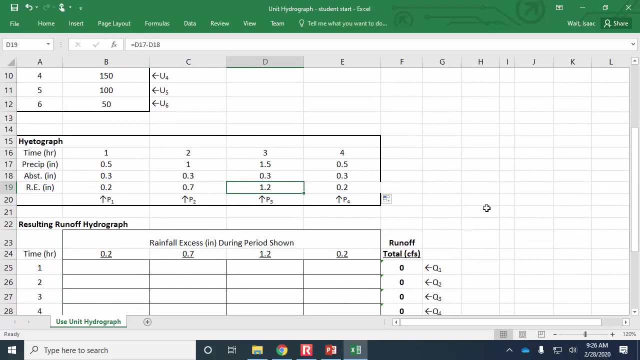 and rainfall excess. specifically, They use P just as the variable, but what they mean is rainfall excess. So rainfall excess during the second hour, rainfall excess during the third, and so on. Okay, now, this is where we linearly scale with the hydrograph that we've got. 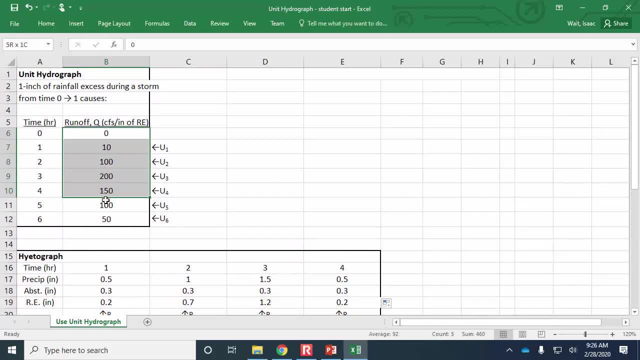 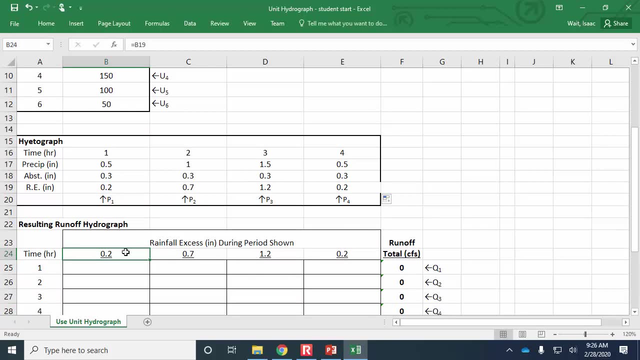 So remember that this is the hydrograph. This is what you'd see from an inch of rainfall excess. How much rainfall excess do we have during the first hour? During hour 1, we only have 0.2 inches of rainfall excess. 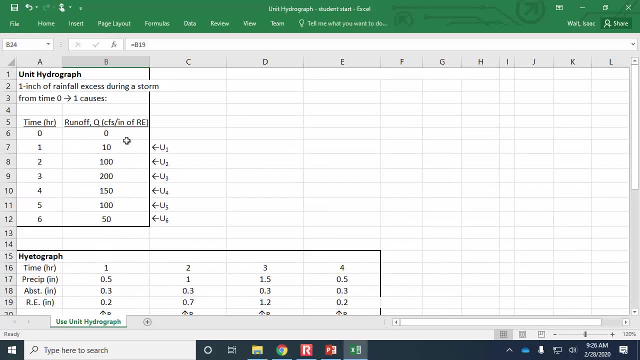 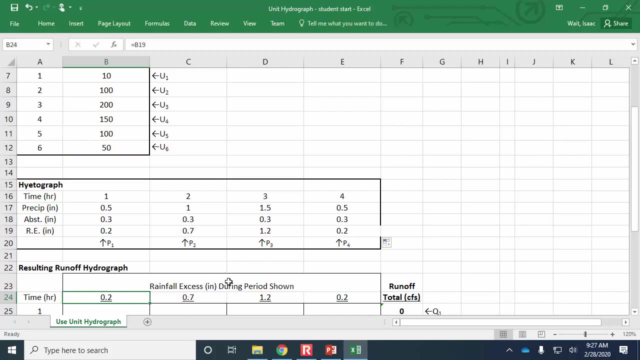 And so what that means is we're not going to see 10 CFS during the first hour, because the units here are CFS per inch of rainfall excess And we only have 0.2 inches of rainfall excess, So the units here, 0.2 is rainfall excess. 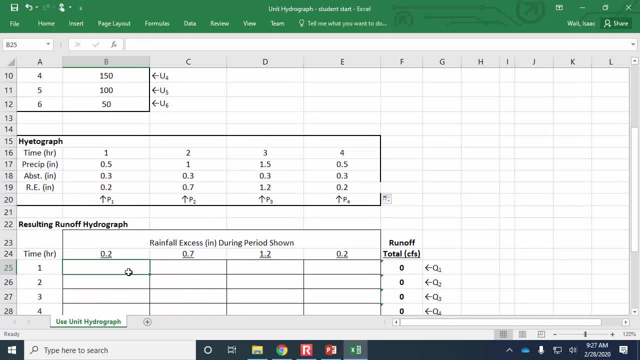 During the period shown. So the way that we do this is: equals the precipitation, the rainfall, excess amount, and you anchor that reference multiplied by the unit, And this is hour 1, so I'm going to go here to hour 1 amount. 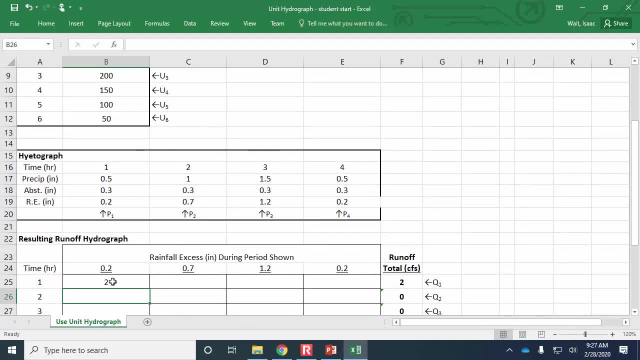 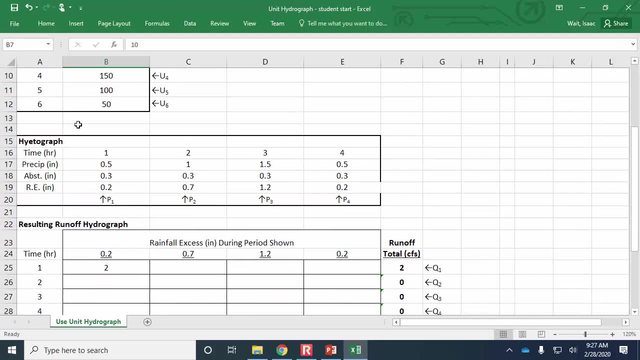 And that's what we'd expect. 2 CFS will come out, because it was going to be 10 CFS If we had an inch of rainfall excess. But we don't have a full inch, We only have 2 tenths of an inch. 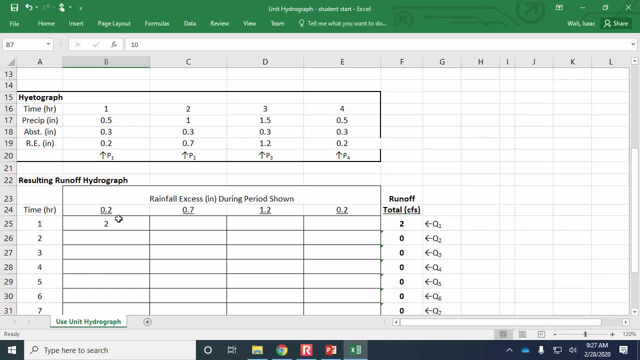 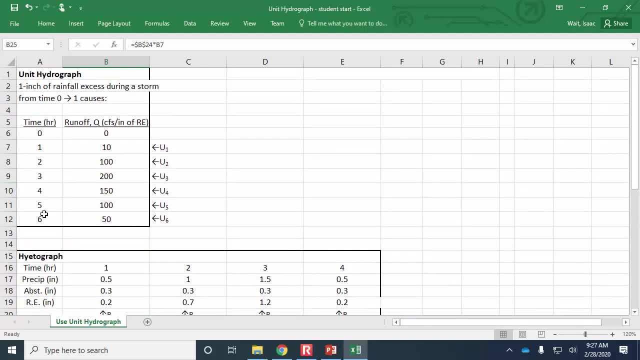 So does everybody understand why it would be 2 CFS? It's just a linearly scaled amount And then we can drag that down And you'll notice that we only have a response through hour 6.. And so I'm going to drag that down through hour 6.. 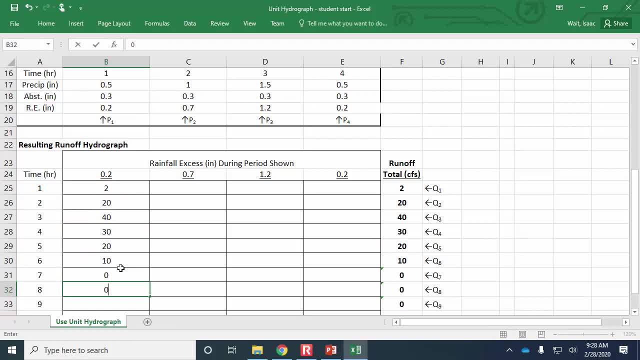 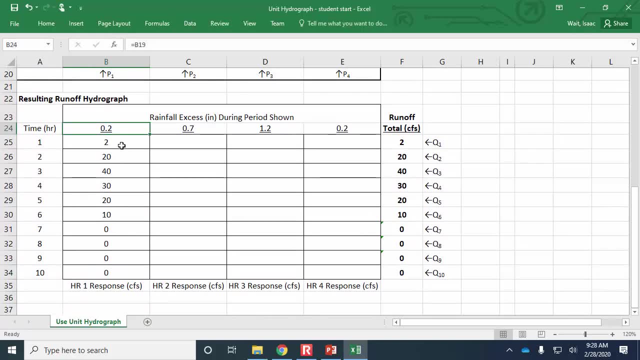 And then afterwards it's just 0 CFS is coming from the watershed In response to this particular pulse of rainfall excess. Alright, now here's where I start to see mistakes when I give quizzes and exams with questions like this. Is that we need to stagger the time? 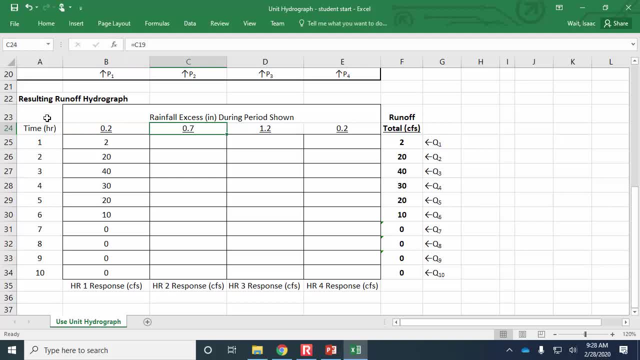 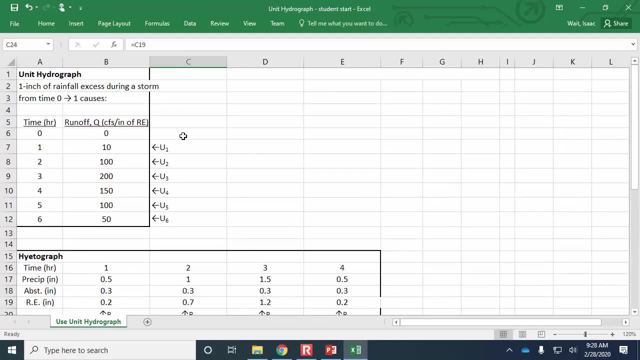 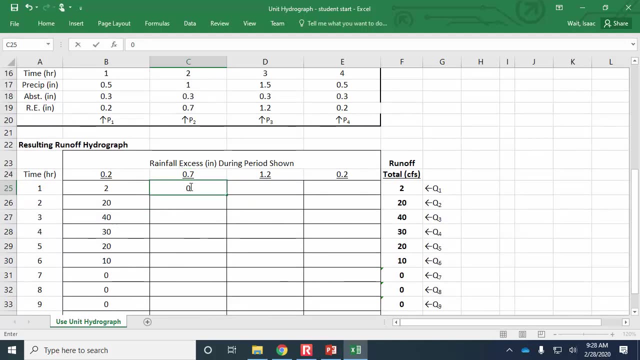 Because, remember, when does this rainfall excess occur? It doesn't occur during hour 1.. This rainfall excess is occurring during the period from 1 towards 2.. So we need to put in a 0 to begin with, To stagger when it happens. 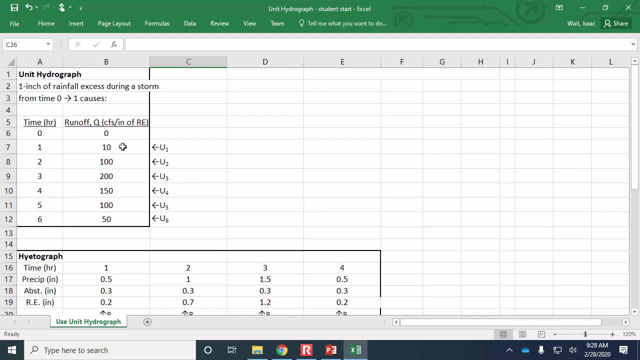 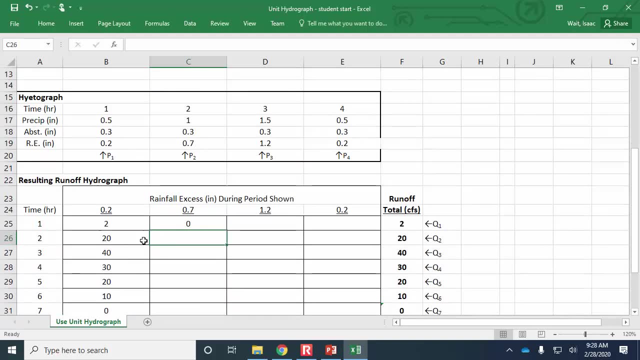 But if it's 7 tenths of an inch of rainfall excess- And we would have 10 CFS for a full inch- Then we should see 7 CFS, But the 7 CFS occurs during hour 2.. So it is going to be this rainfall excess amount. 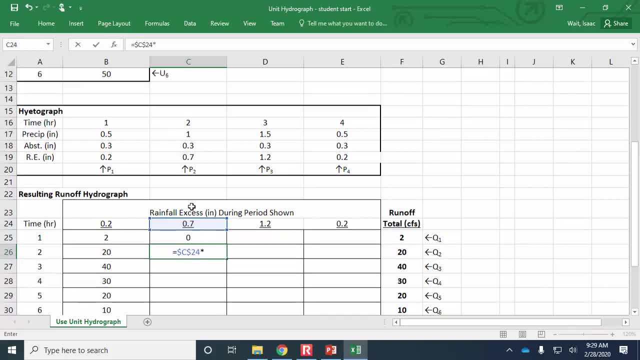 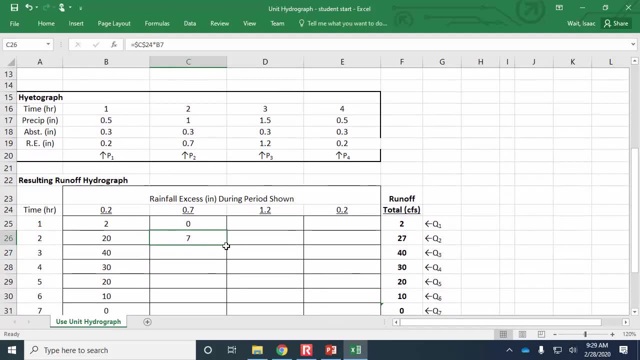 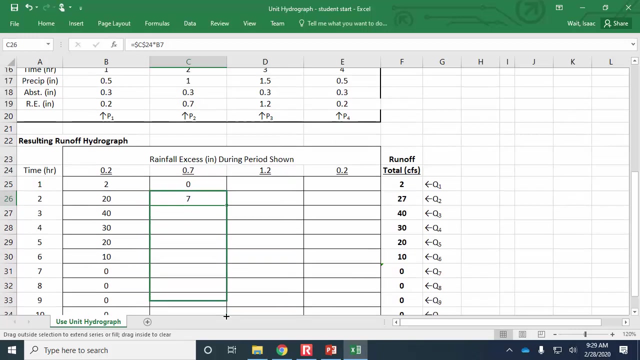 Anchor: the reference Multiplied by the unit hydrograph, The unit hydrograph. But what you'll see is that the 7 CFS comes during the second hour, Because this rainfall was itself during the second hour, And then the watershed response to that occurs through the 7th hour. 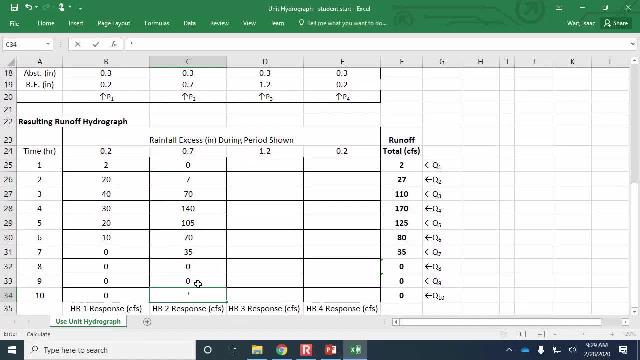 And then afterwards there is 0 CFS. Okay, so I'm going to pause the recording And give you some time to apply that same method For the third hour And the fourth hour, And I wish I had remembered to delete this formula over here. 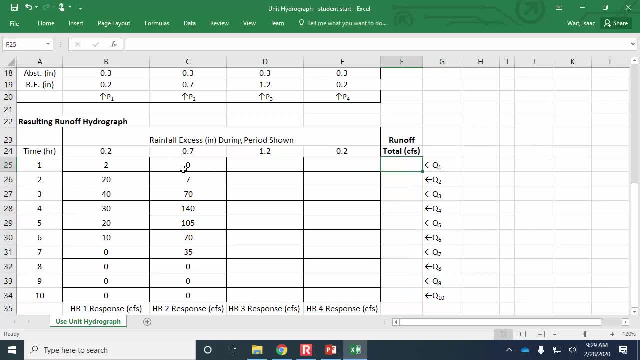 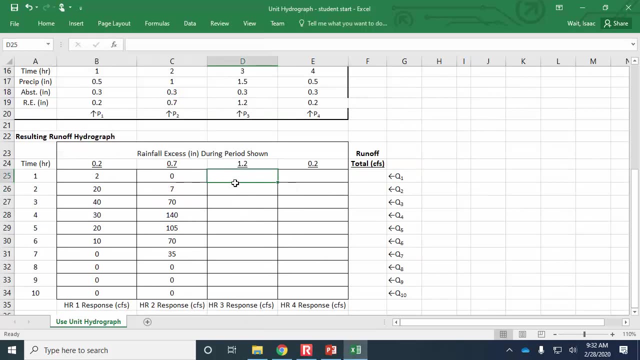 The total is going to be the combination of all of these four periods that are to the left. So let me give you time to work on that independently, And then we'll see if we all have the same runoff amounts. So for the third hour, 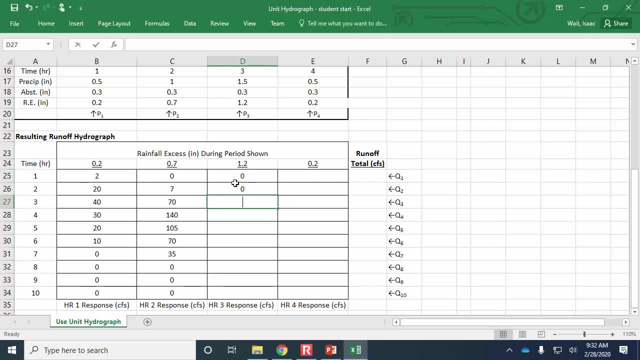 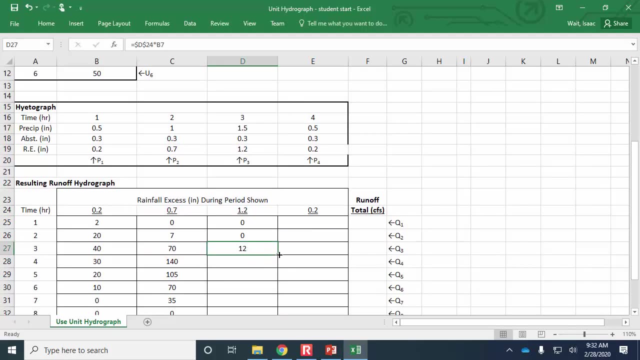 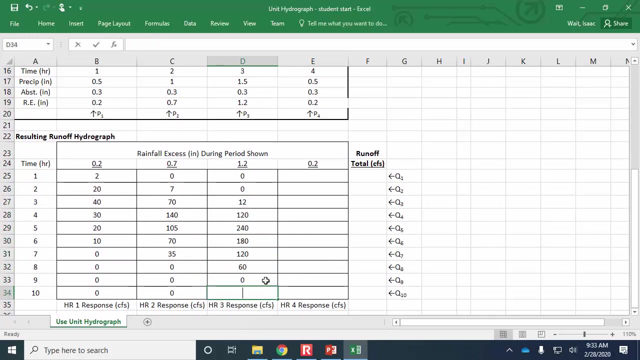 You need to put in 2 hours of delay And then begin the response of the pulse of rainfall excess Multiplied by the response, And then dragging that down through The 8th hour And then for the last, We have 3 hours where nothing occurs. 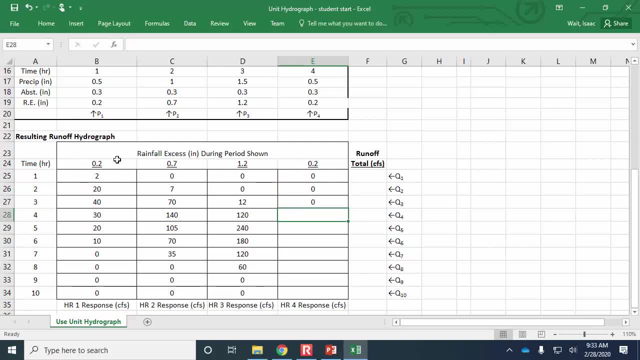 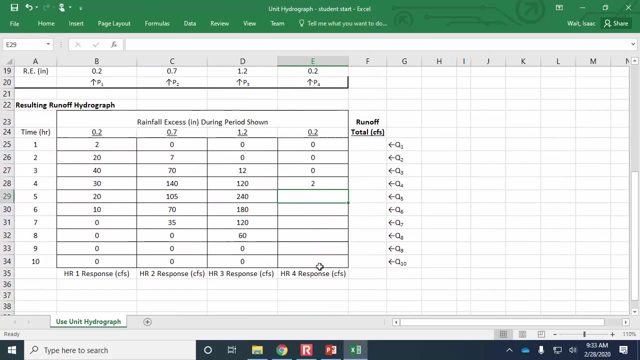 Because this 0.2 inches of rainfall excess comes at the end of a sequence. So then, in the fourth hour is when we begin to see the effect of that, And at first is going to occur over the area that's closest to the outlet. 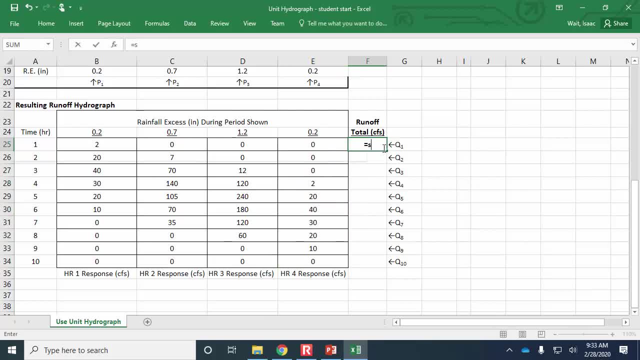 So the totals will be The combination of all of the pulses of rainfall And so if we look here in the middle, This 385 CFS, What it means is that at a certain time You're seeing the tail end of the first pulse of rainfall excess. 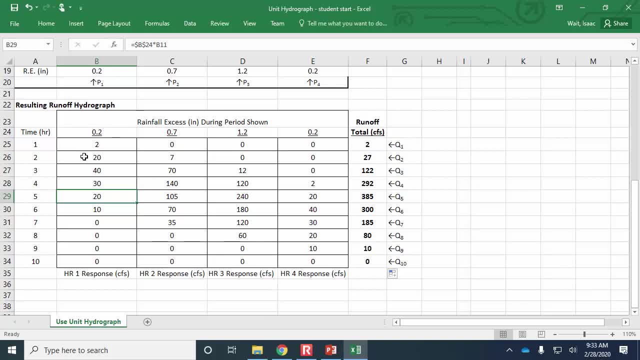 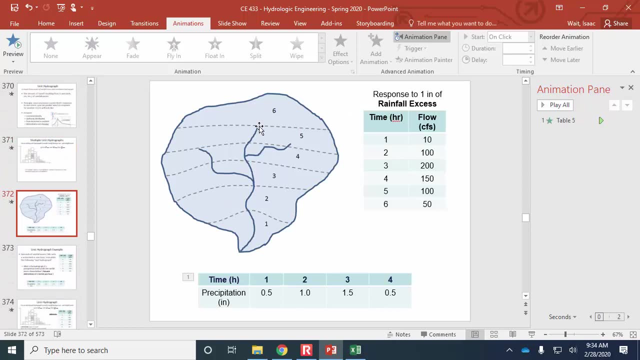 The 0.2 inches of rainfall excess is mostly through the system. What we're seeing at time 5.. Is that contribution at the furthest part of the watershed? So if we look at the diagram, It's the rain that fell over here. 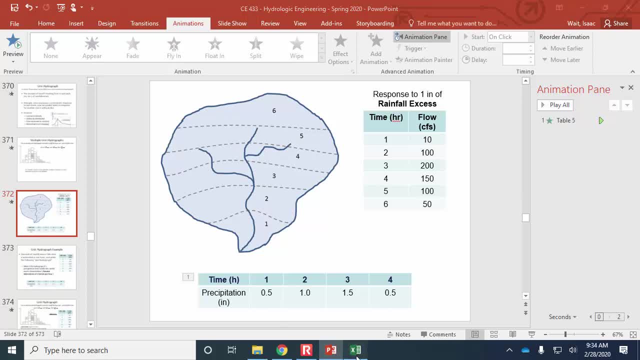 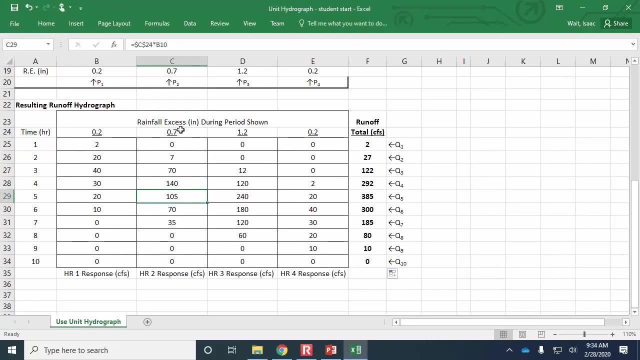 That's finally now just making its way to the watershed outlet. Combined with the rainfall, that The 0.7 inches of excess. That is not as far through the cycle. You know this is at the middle Of the cycle, Whereas this was at the tail end. 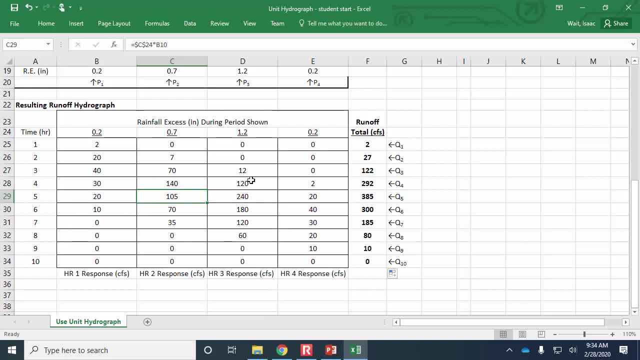 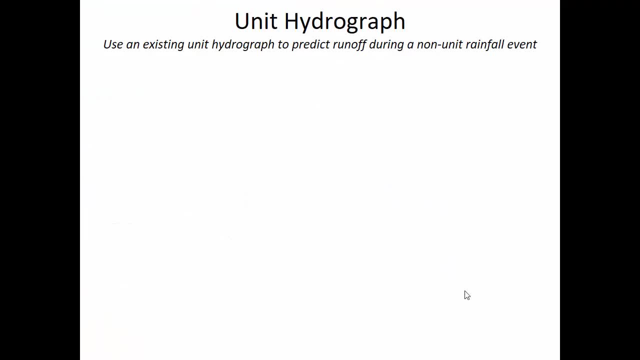 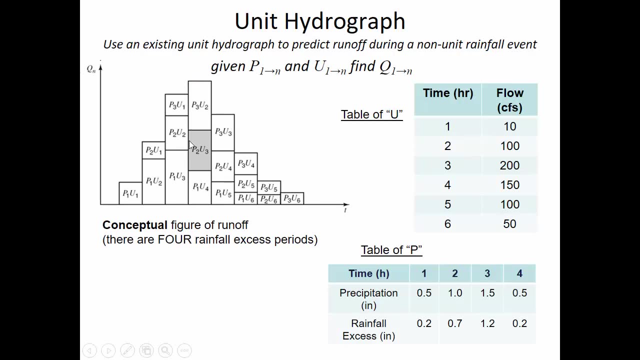 And it's the combination of all of them, And so This figure that is showing the equation for it. What it illustrates is that The highest peak Is going to be the precipitation that fell during the first hour Acting over A further away area. 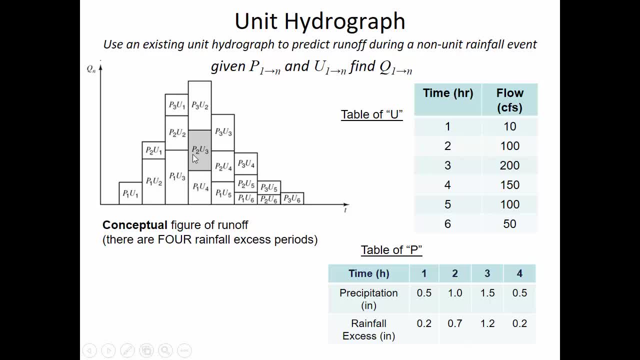 So this just saying area 4.. And the precipitation during the second time period Acting over area 3.. The precipitation in the third time period Acting over area 2.. And so This Formula For a runoff hydrograph Is kind of built into the spreadsheet structure. 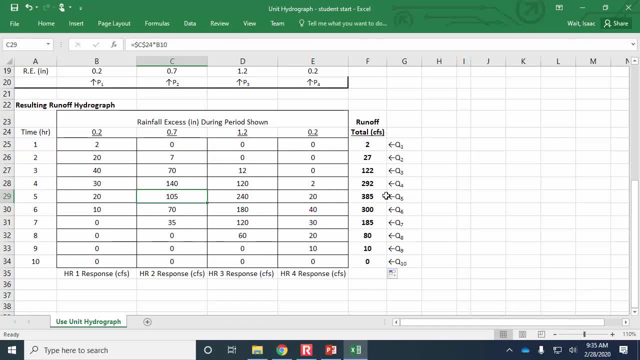 Where you're adding it up. Each one of these Cells Is the effect of P1., U5., P2., U4., P3., P4., P5., P6., P7., P8., P9.. 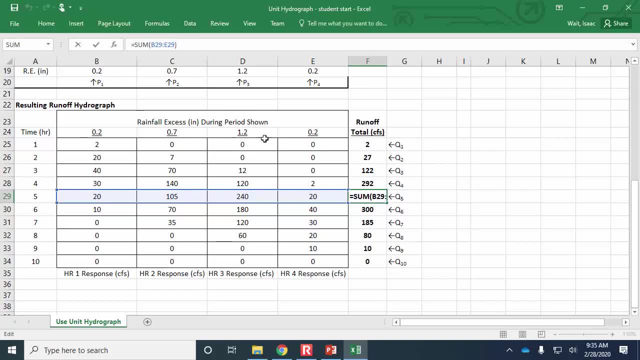 P11., P12., P13., P14., P15., P16., P17., P18., P19., P20., P21., P22., P23., P24., P25., P26., P27. 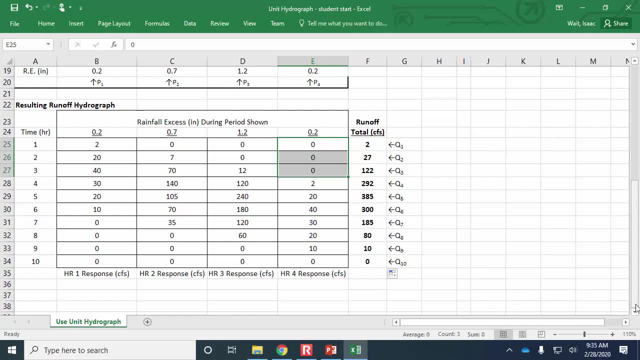 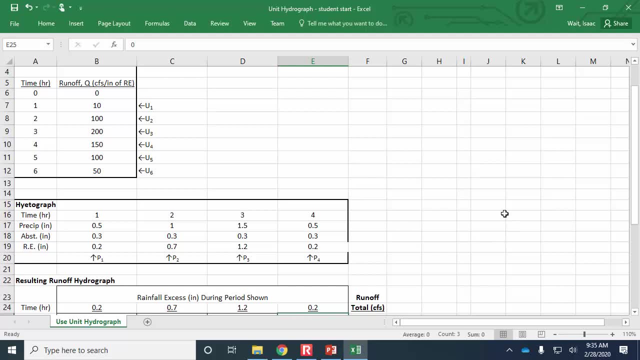 P28., P29., P30., P31., P32., P33., P34., P35., P36., P37., P38., P39., P40., P41., P42., P43., P44. 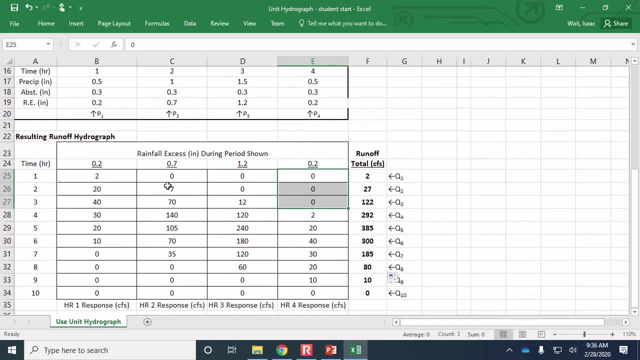 P45., P46., P47., P48., P49., P51., P52., P53., P54., P55., P56., P57., P58., P59., P60., P61., P62. P63., P54., P56., P57., P58., P59., P60., P61., P62., P63., P64., P65., P67., P68., P68., P69., P70. P71., P72., P72., P73., P74., P74., P75., P68., P78., P79., P78., P79., P80., P81., P82., P82., P83. 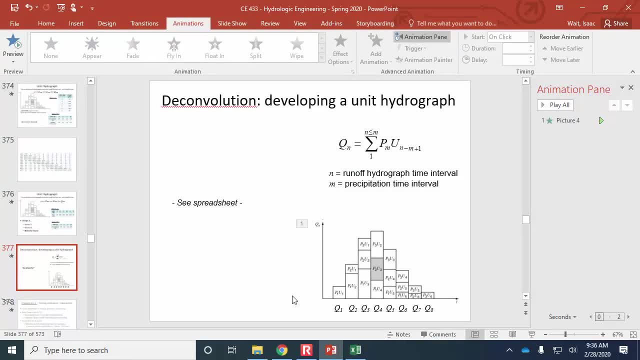 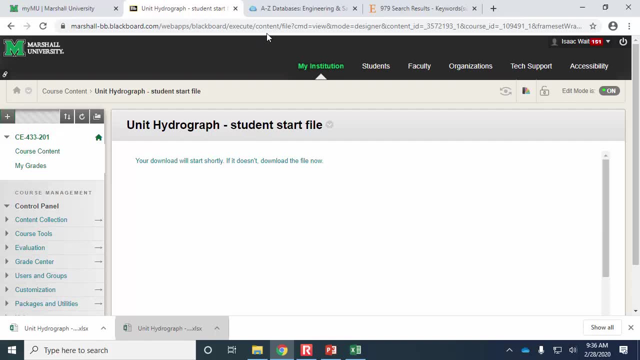 P54., P54., P55., P56., P57., P58., P59., P59., P60., P60., P61., P62., P62., P63., P64., P65., P65. P67., P68., P68., P69., P70., P70., P71., P72., P72., P73., P74., P74., P75., P68., P78., P79., P70. 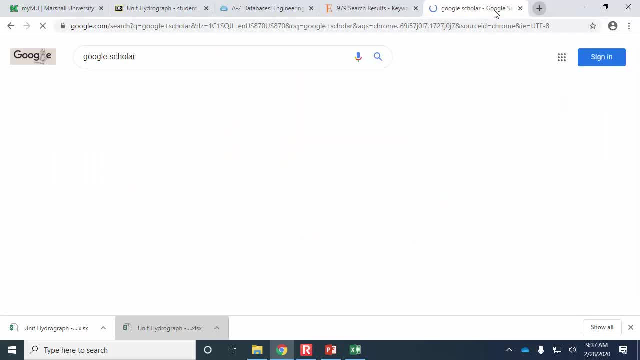 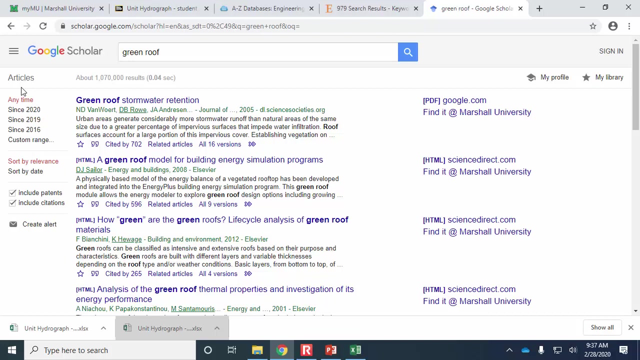 P71., P61., P62., P72., P61., P72., P, journal articles. but one of the things I want to point out is that the more citations an article has, you can think of that as an indication that it's more. 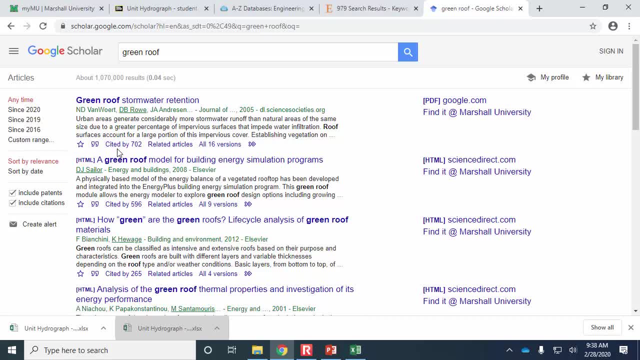 important and impactful and authoritative and so, for example, with 700 citations for this particular article, it's probably a really good one. it's one that lots of other people have referred to as kind of seminal, and so the cool thing is is that I think Google consents that we're at Marshall and 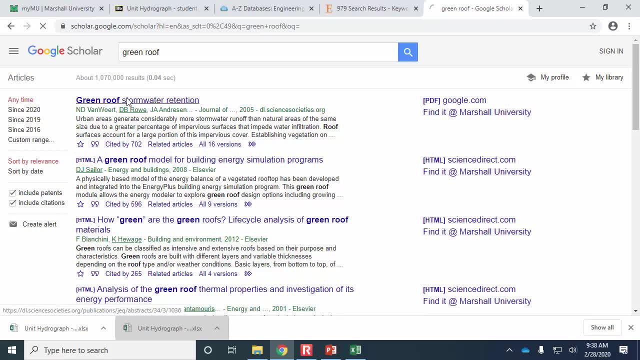 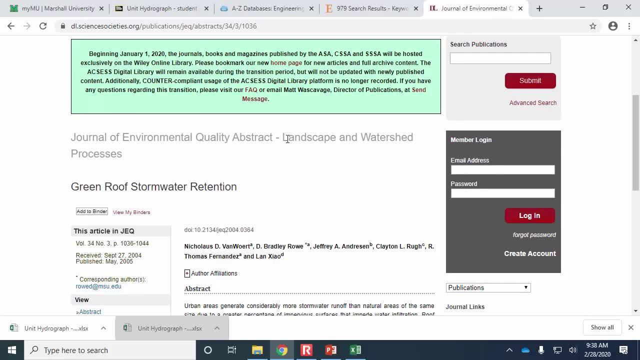 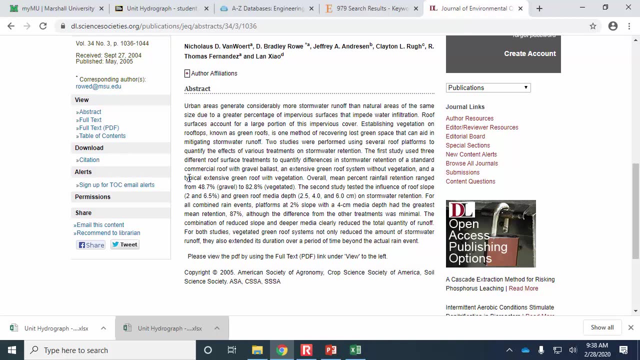 it'll go and help you find the article. so if we just use this one as an example, I'm not sure if we have access to the Journal of Environmental Quality text to the left. let's see if we get the full text in that one. okay, not through that. 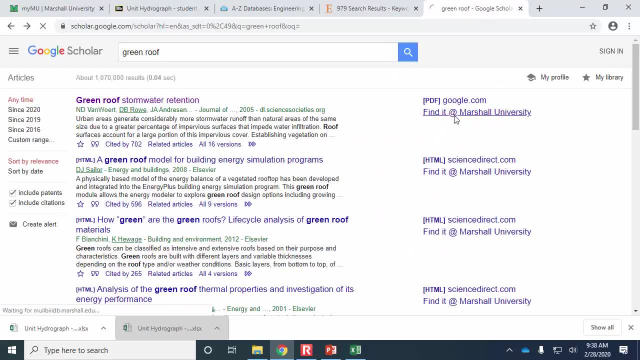 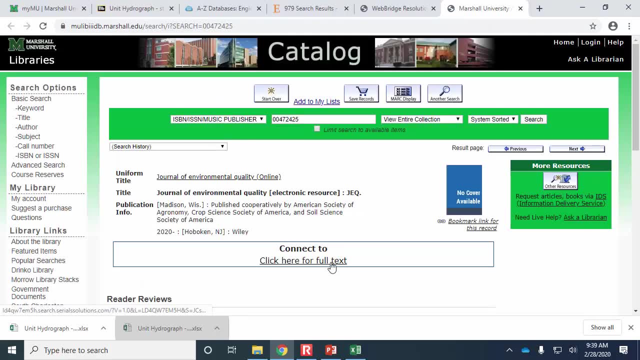 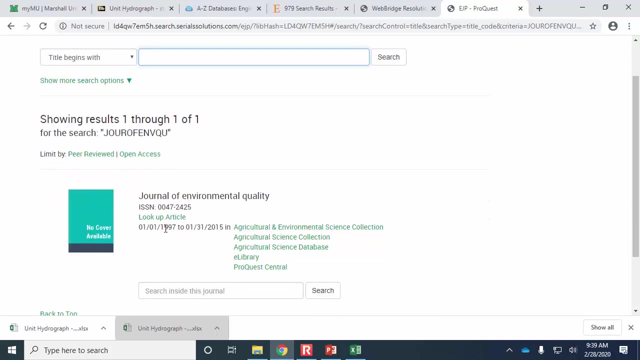 but if we do the find it at Marshall University looks like we can get the full text, so this link will find it. on the library catalog, the Journal of Environmental Quality, we've got it from 97 to 2015 and this particular article, I think, was from 2005, so 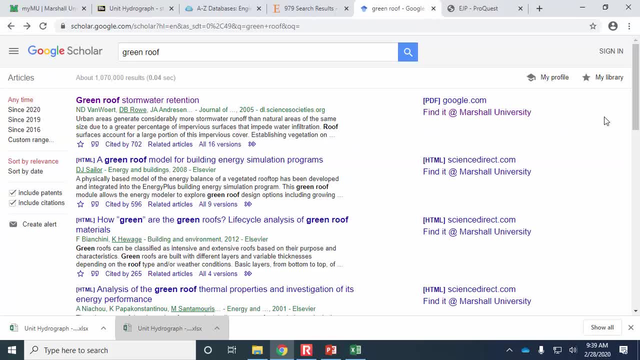 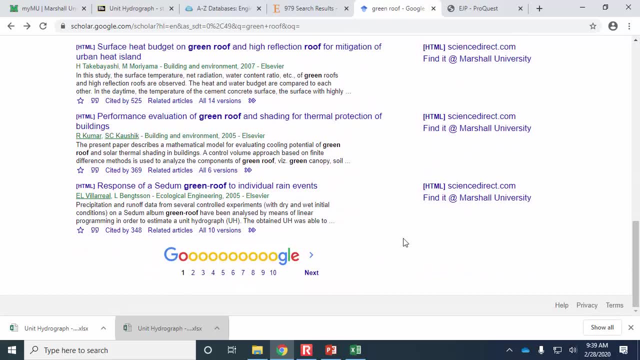 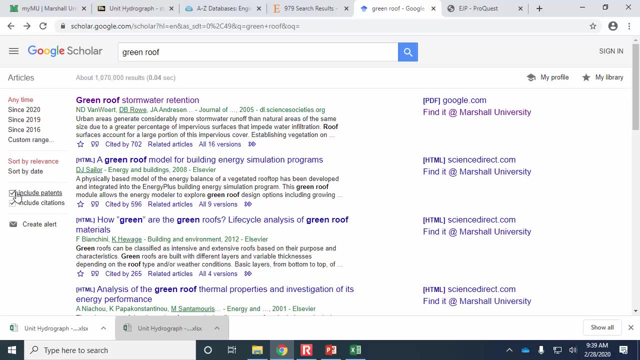 Google Scholar is maybe the most streamlined and I like it, especially because you can find out now how highly cited particular articles are. and for this particular topic of green roof, you see that there's a million articles. so even if we exclude patents, that's still more than 900,000. you'll notice right now. 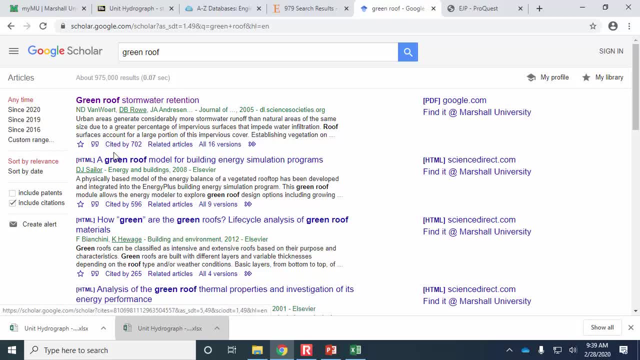 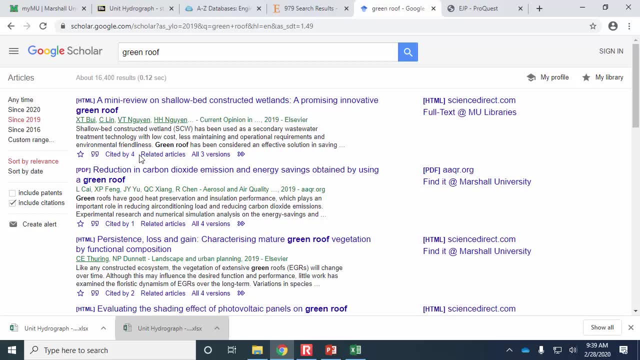 we're sorting by relevance and so it's going to have the most highly cited articles first. but if we just screened that, we only want to see maybe the articles from last year and newer, there are going to be fewer citations because it's just been in. 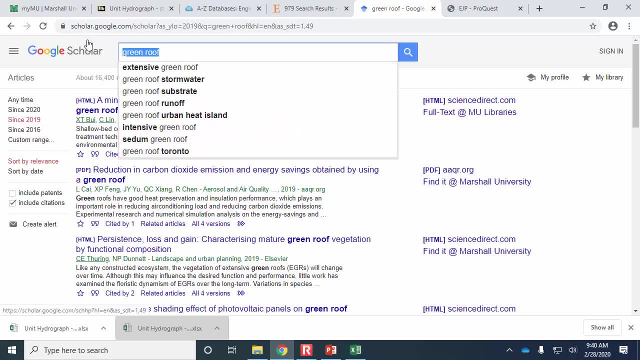 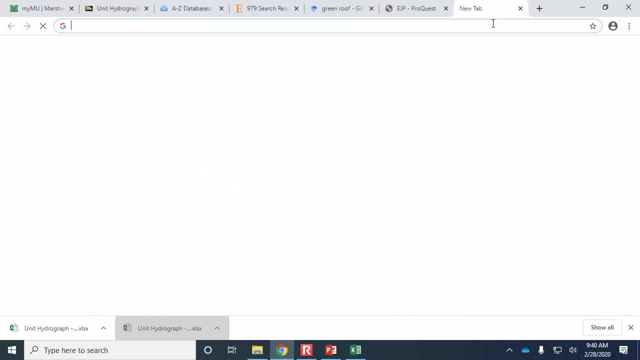 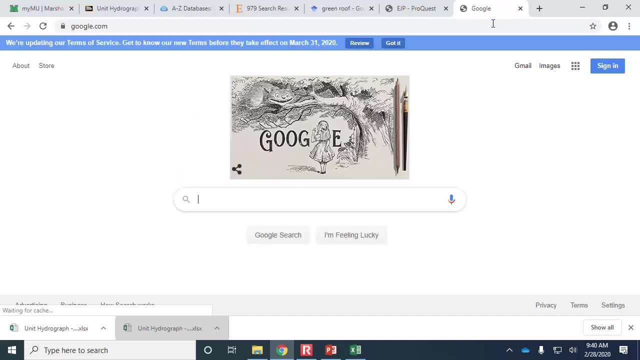 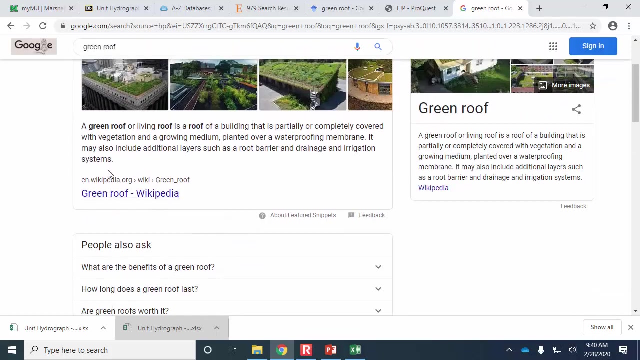 the literature, less So any one of these topics. I think Google Scholar would be a good place to start. It's going to be better than just a Google search, because if we go to Google itself and not Google Scholar, Wikipedia is the first response and I mean it's fine to. 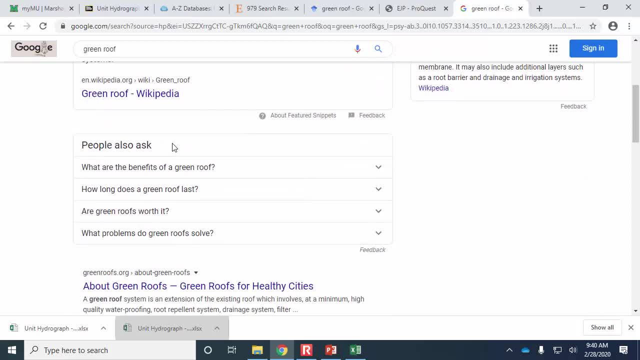 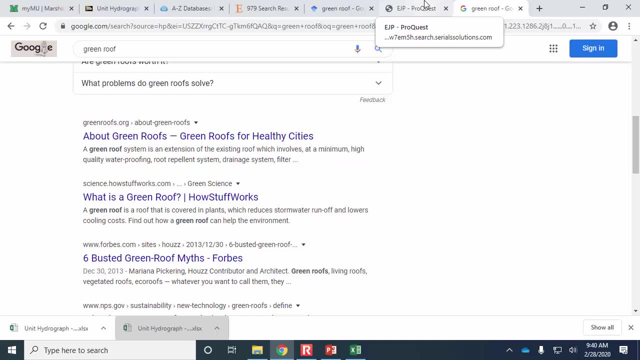 read Wikipedia so that you get a better understanding of a topic- Greenroofsorg. it's just not as authoritative and for a technical writing assignment like this busted Greenroof myths anytime. There's a number like this. it's just click bait, right? They're hoping that you'll click. 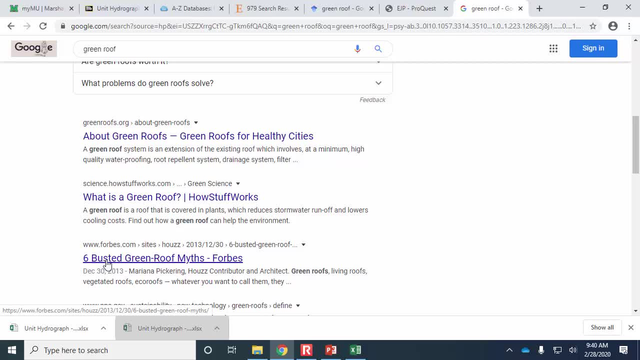 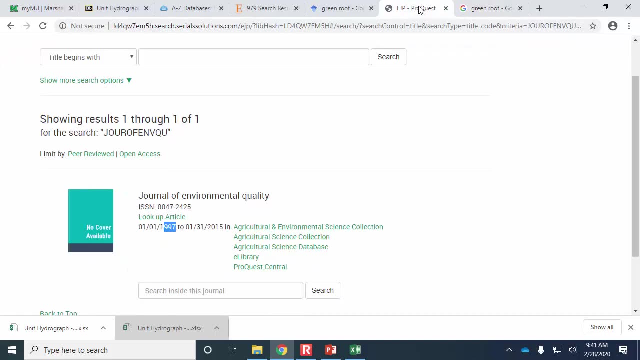 on the next thing and they're loading a bunch of commercials in between. It's like a salacious headline busted myths. you know six things the doctor doesn't want you to know. Your electric company will be so angry if you learn this information. So the more important stuff: 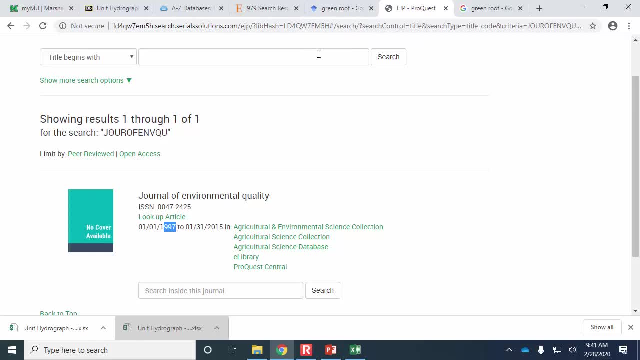 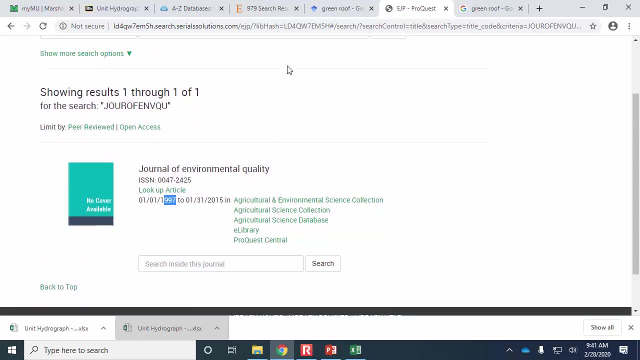 for a research paper you're going to find through scholarly journals, and so it's peer reviewed. And what peer reviewed means is that before this paper gets published, they'll send it out to three or four other researchers who try and find mistakes. They'll ask questions. 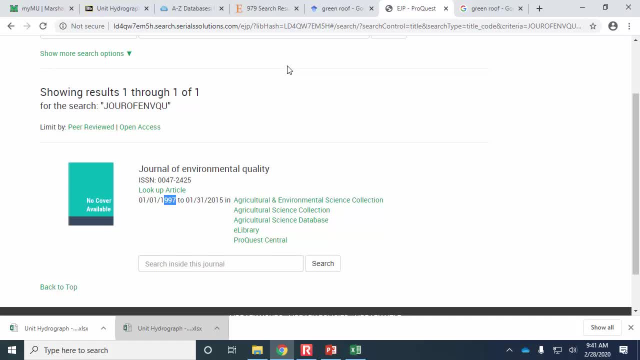 related to the research methods. They'll see if they can contradict the results and the conclusions that the authors have come to, and they basically try and throw rocks at the articles. So by the time it gets through that peer reviewed process, they hope that they've been able to weed out the information that they're trying to find, And so that's. 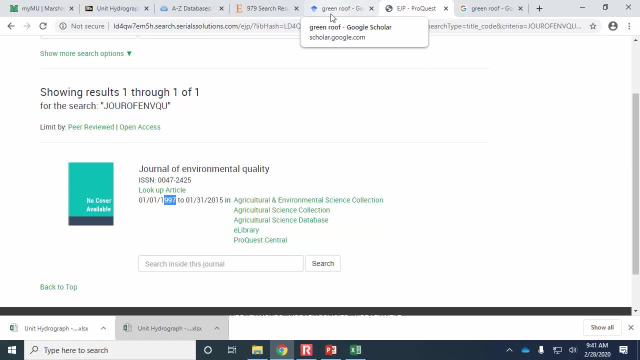 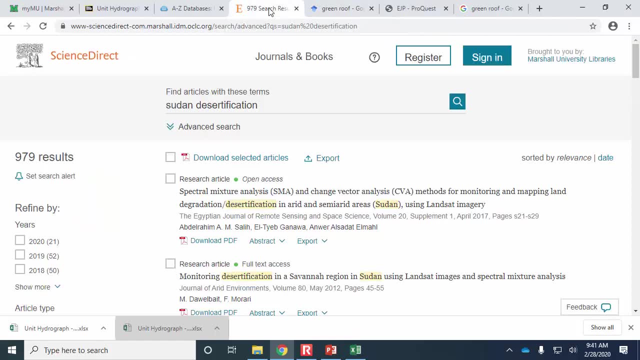 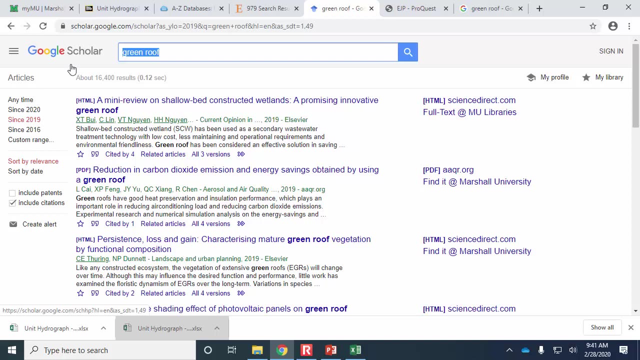 what they're trying to do. They're trying to weed out papers that had a conflict of interest, papers that weren't based on meaningful data, And so you can just kind of take it as a little bit higher quality. So my suggestion is that you know you use Google Scholar as one option and then on the 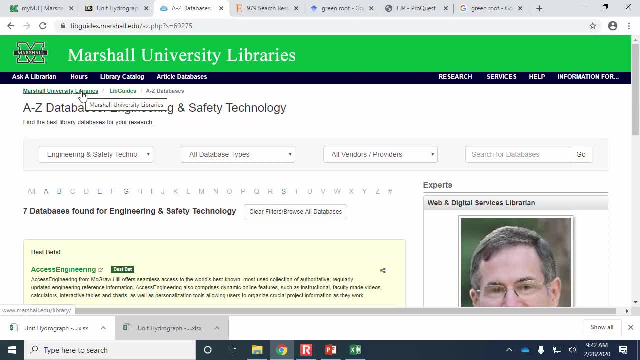 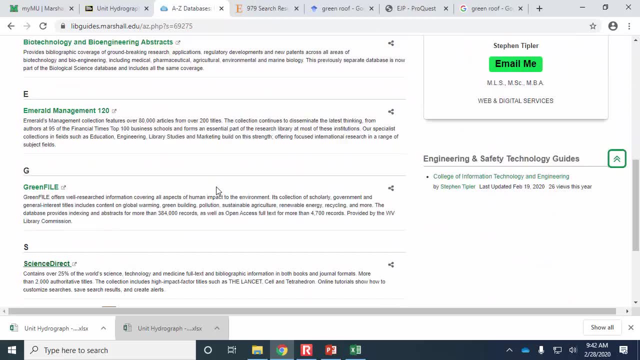 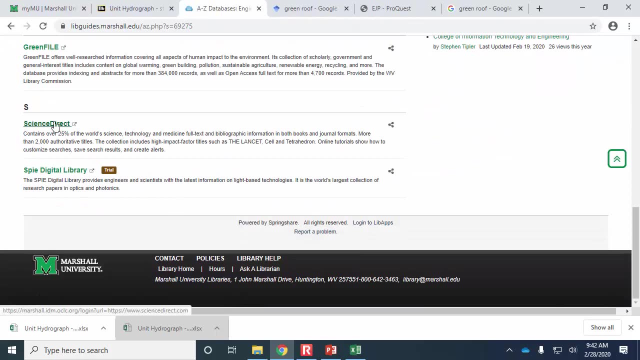 Marshall Library's website. they have a series of databases. Access Engineering is a good database, And ScienceDirect is another one that I've used quite a bit, And so I've got ScienceDirect up right now. So let's just take a look at how we would get information through ScienceDirect. 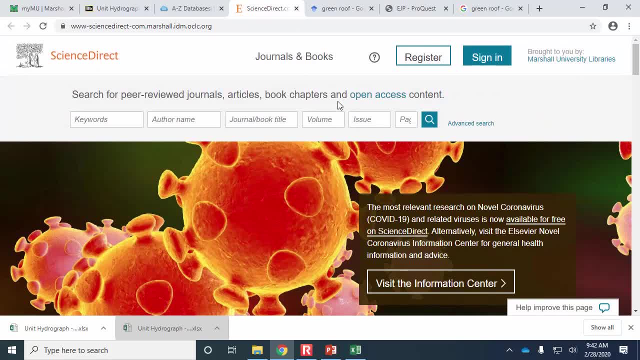 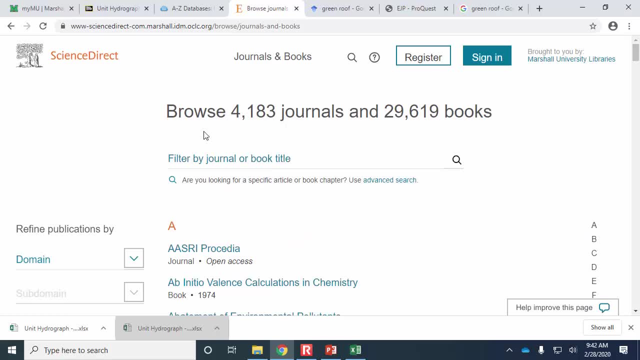 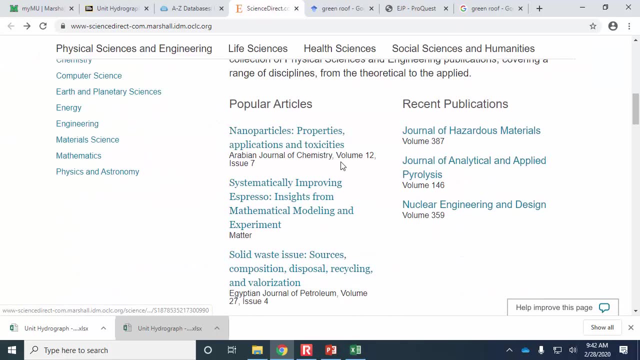 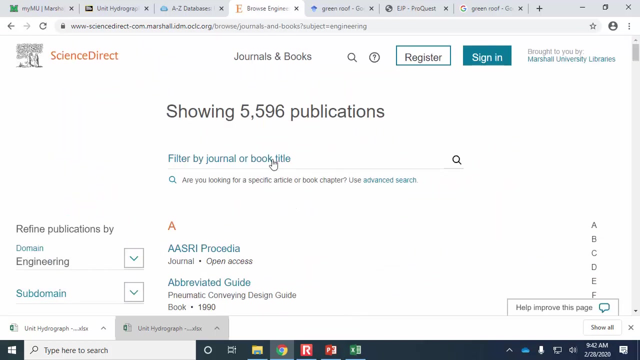 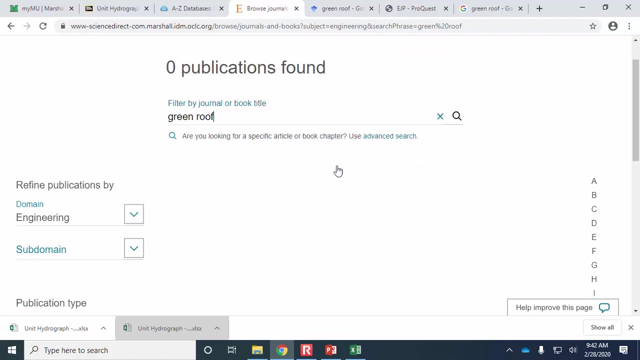 In ScienceDirect there is a search tool And I'm going to search it by topic. So I'm going to search by topic, not necessarily by the journal itself. Okay, yeah, So over here, if we would choose Engineering, then we'll try Green Roofs again. Let me do the 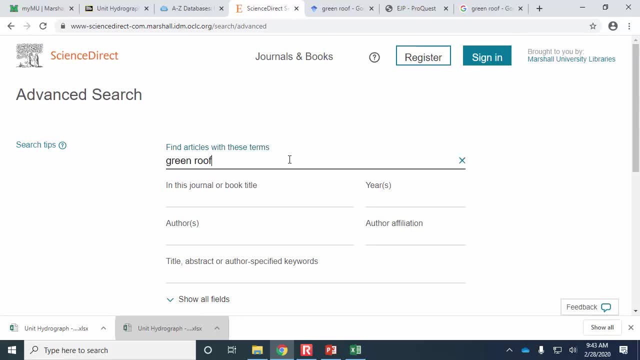 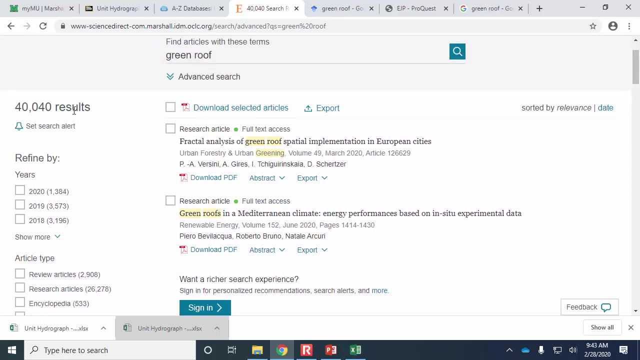 advanced search Articles with these terms: Green Roofs. All right, So it's brought up 40,000 results, So I'm going to do a little bit more research here. So I'm going to do the advanced search And again, this is one of the research agencies. So you need 16,319. 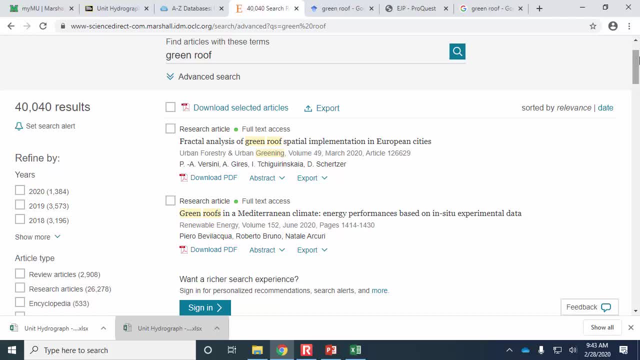 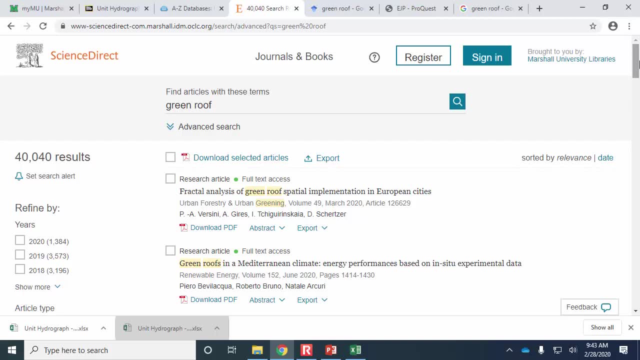 less results as opposed to the 900,000 in Google Scholar, because what it's identifying here is just the journals that indexes in ScienceDirect And I think it's like a family of publishers that are all aggregated the indexing together, But it looks like we would. 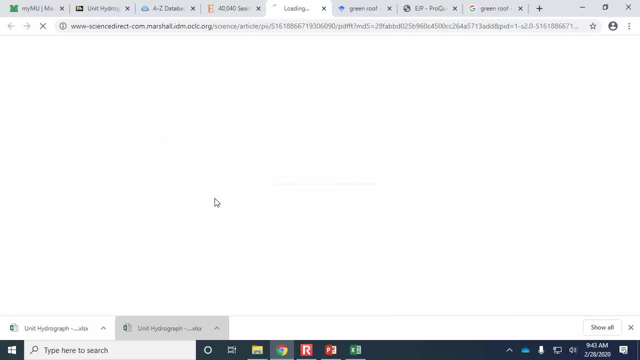 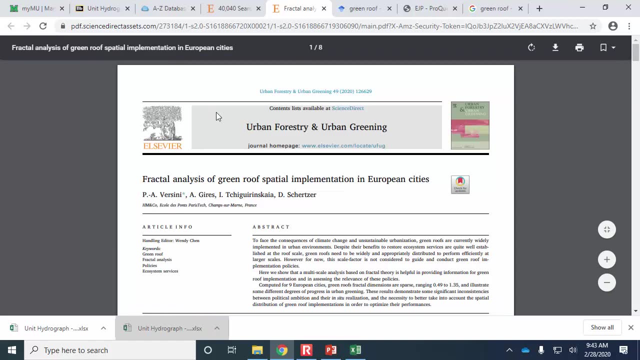 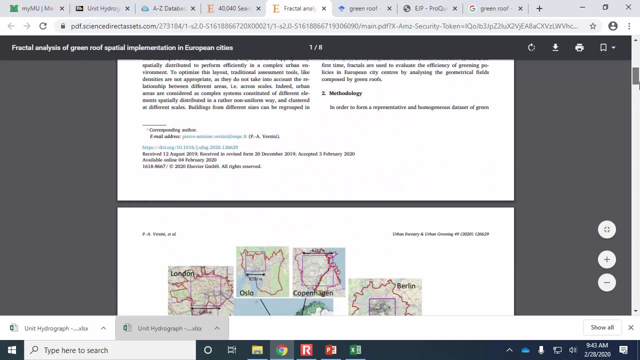 have the same kind of full-text access here that we could get with Google Scholar, linking through the library ichen زarios clic so o temas. ask that you include the full citation information, like the authors, the title, the name of the journal. Here it's showing the issue number, the page number. So I think, if you begin now, 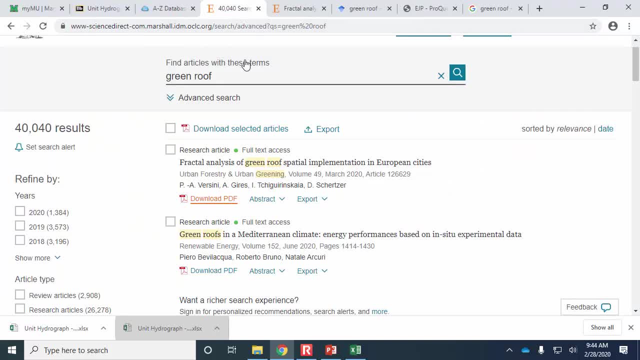 the assignment is that you should have ten references to peer-reviewed papers. It's going to be really easy to find ten papers out of 40,000 that are worth citing. So if you begin the research now, then you can read through them and kind of identify what are the statistics. 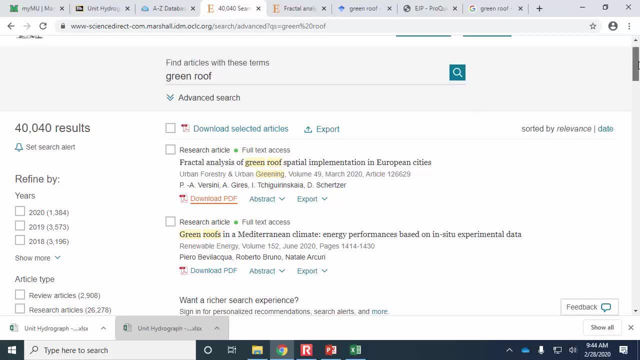 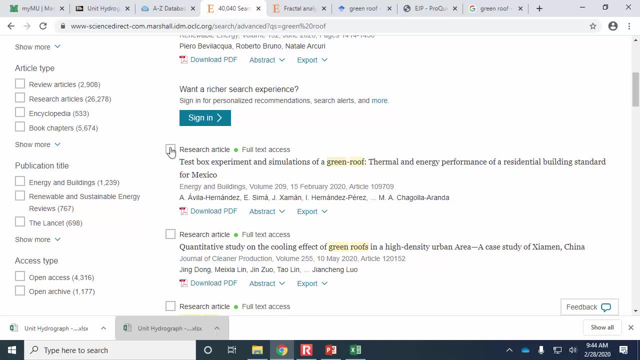 that you want to cite, or what are the main pieces of information that you're interested in including for the research paper. If you have any questions about other project topics, then let me know and I'll be happy to see if I think it would be a good one for this. 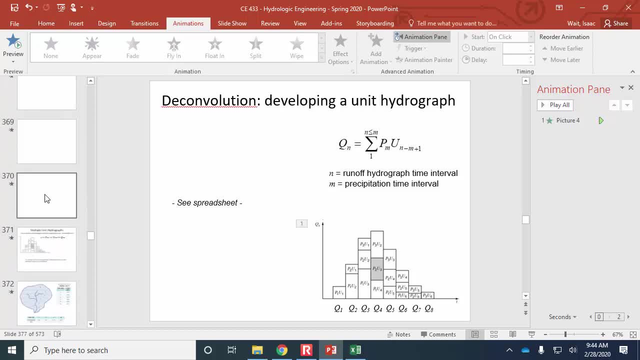 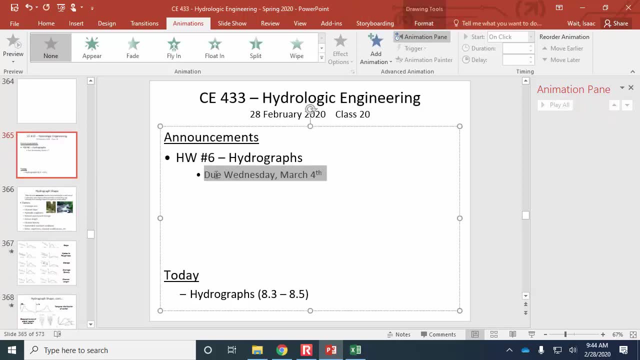 particular assignment. Before we finish a couple minutes early, let's just take one last look at the announcements. I think all it says is that the homework assignment is due on Wednesday. So now that we've done the unit hydrograph stuff, I'd encourage you to get started on that early on, And that's.